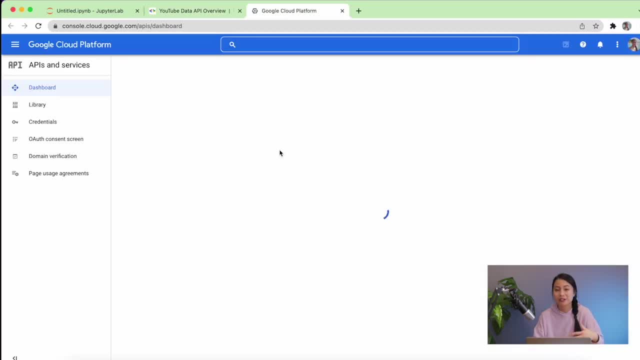 Let's click on the Google Play button. Let's click on the Google Play button. Let's click on the Google Developers Console link. If you have a Gmail account, you should have access to this website. I'm already logged in, so this is my Gmail account. Then create a new project by clicking. 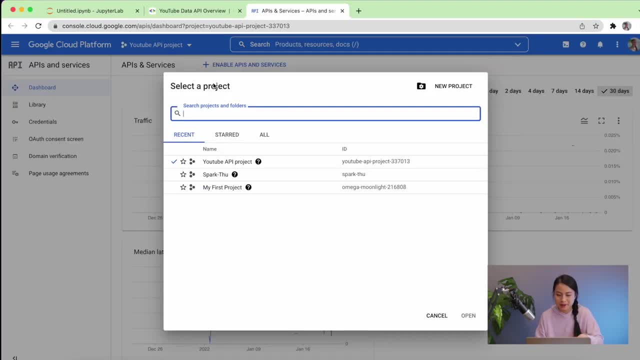 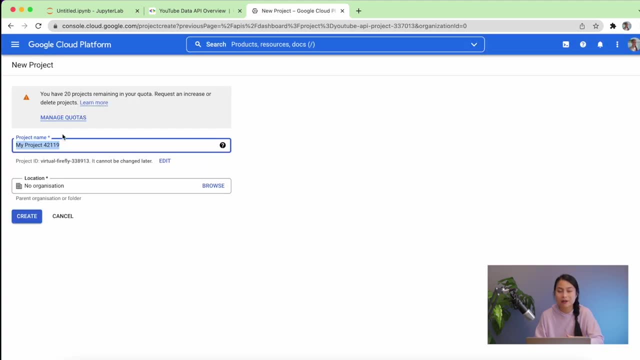 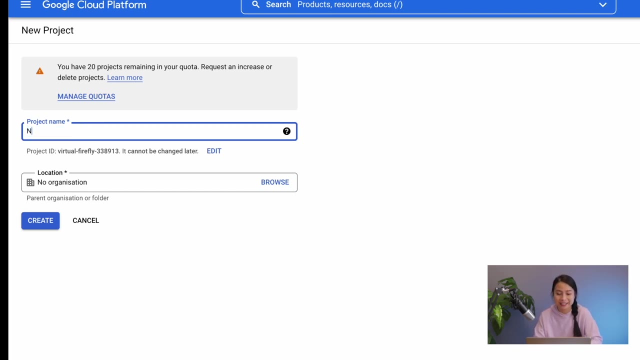 on this button over here You might see a different button. if you don't have any project yet. I already have some projects, but let's just create a new project, just to show you how it works. Now let's create a new project and let's choose a project name, Just let's say new project. 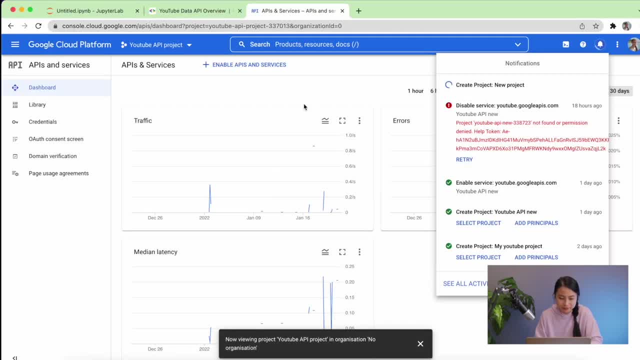 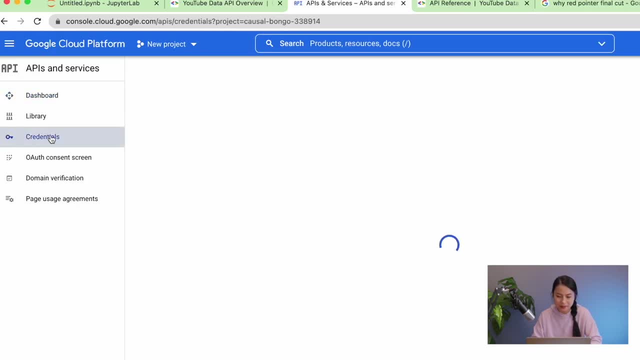 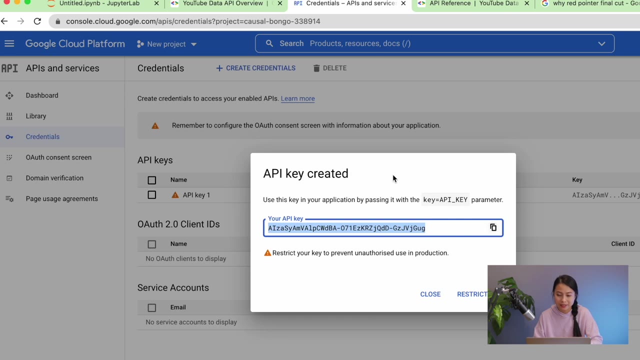 Let's click on create. Next, we'll need to request an API key by clicking on the credentials section over here, Then create credentials. Now we have the API key and we just need to copy this API key into our notebook. Let's quickly do that. As you can see, an API key is just a simple encrypted string that identifies as an applicationoras, and I'm limited to a single present string with定p. If you click on this monkey arrow, you can see that the key has been created and typed into the API key function. 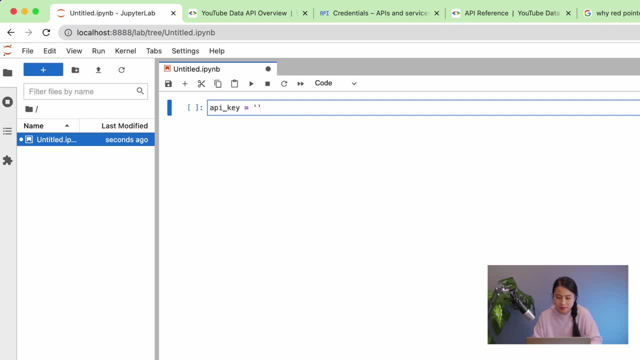 As you can see, an API key is just a simple encrypted string to edit in addition to semana Email. So we can create an API key page or a single session page page. Just specify any lässt должна dans. what we know is our API key, because API keys are going to have to edit files in Faculty. 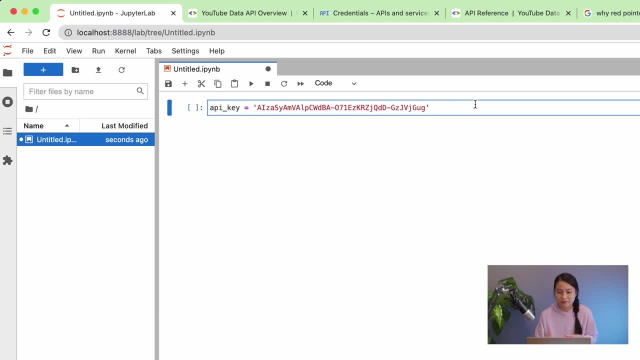 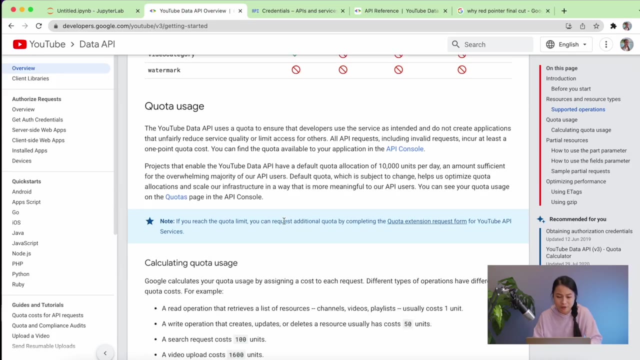 api key is just a simple encrypted string that identifies an application. so it's used to associate api requests with an application for billing and quota and etc. so if you scroll down over here in the documentation, you see that the quota limit for youtube api is 10 000 units. and how many units you? 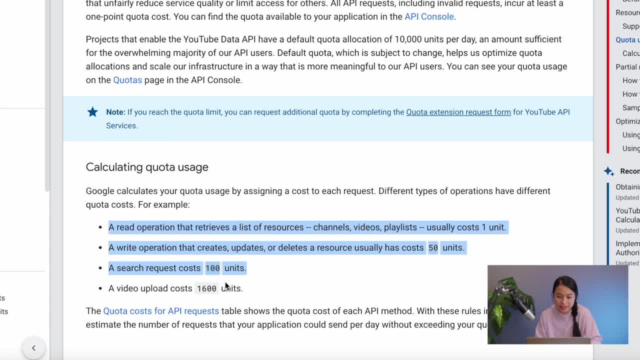 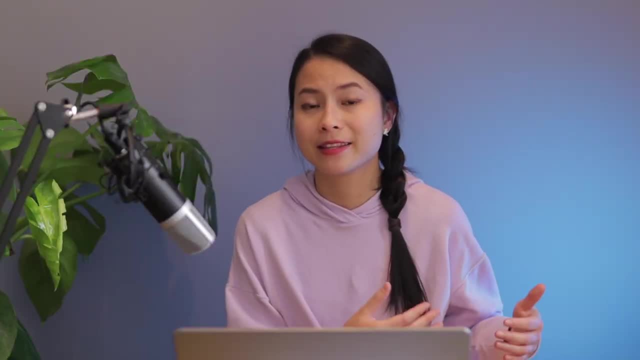 use depends on what kind of operations you're requesting. so the read operation, which is what we'll be using, is actually very cheap. it's only one unit per operation. but the right search and video upload cost a lot more units. so this limit is to prevent that some applications will make. 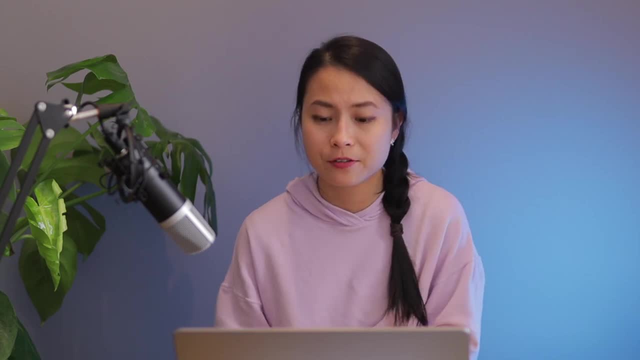 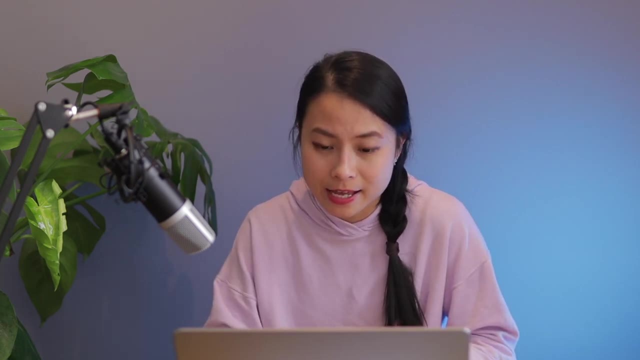 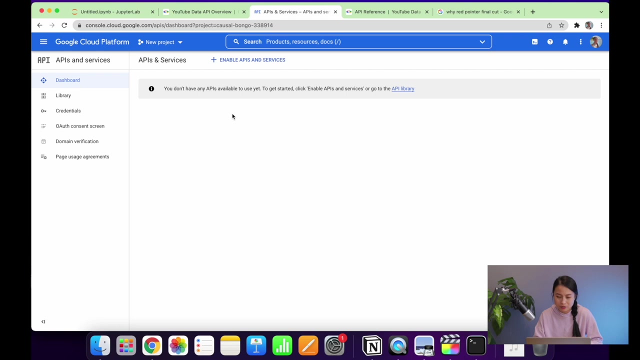 too many requests to the api server and overwhelm the server, and other people cannot request any data anymore. the last step we need to take for the api access is to enable youtube api service for our project. let's go back to the dashboard in the google developers console, click on enable apis and service button. then we can search for the. 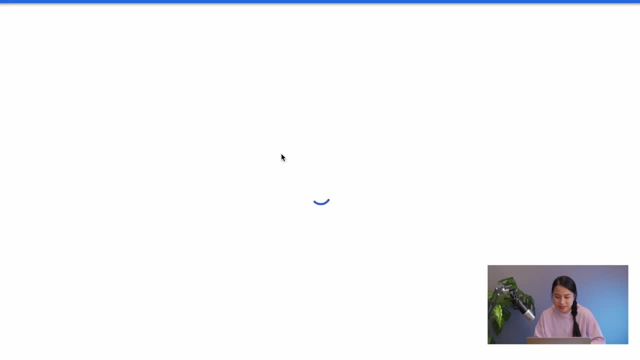 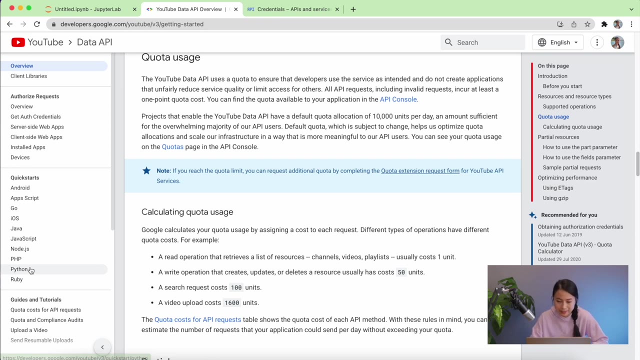 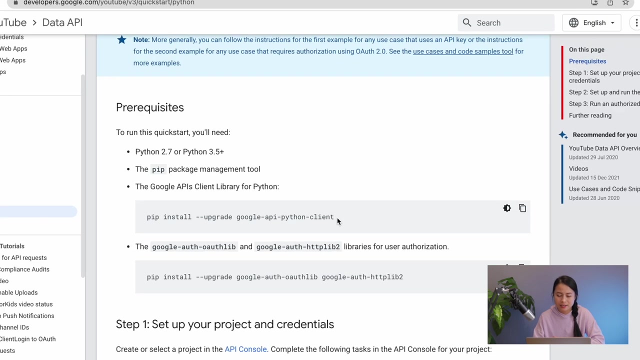 youtube api version 3. and here it is. click on it then enable done. now under the quick starts tab in the youtube api documentation page, we go to python. because we are working with python, we can see the required packages in order to use the youtube api. we just copy this code into our 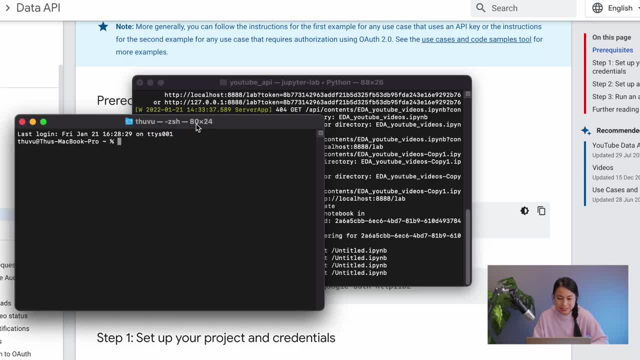 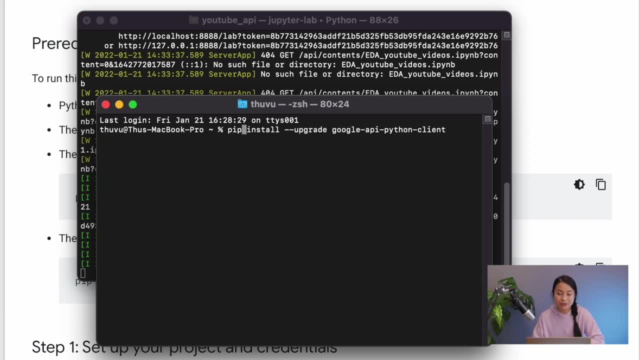 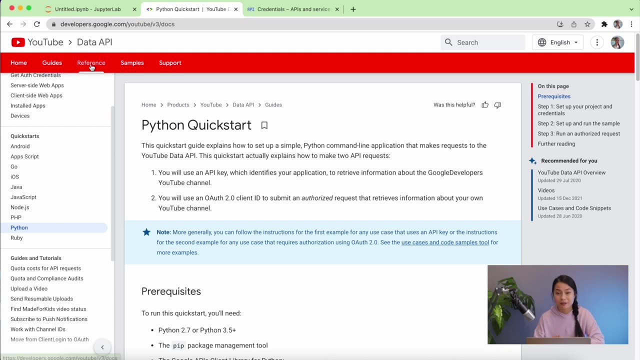 api and we're going to install these packages. the package we need to use is the google api python client package. i'll just copy it here, because my macbook also has python 2 installed, so i'll need to use pip3 instead of pip. now let's dive into the youtube api references to see how to use it. 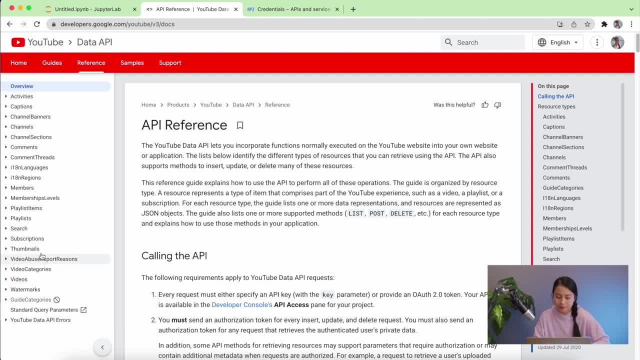 on the left. here is all the information that we can request with the youtube api for retrieving youtube video data. we'll look at three modules: the channel name and the channel name and the channel is module. the playlist items module and the videos module. we all know how youtube works, right? we have 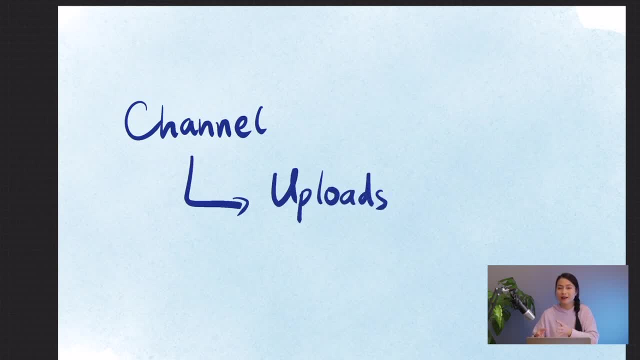 the youtube channels, then we have the upload playlist and then under this, this upload playlist, we have all the videos. so if we have a channel id, we can find out what is the upload playlist id of that channel and from this upload playlist id we can find out all the video ids of this channel. and 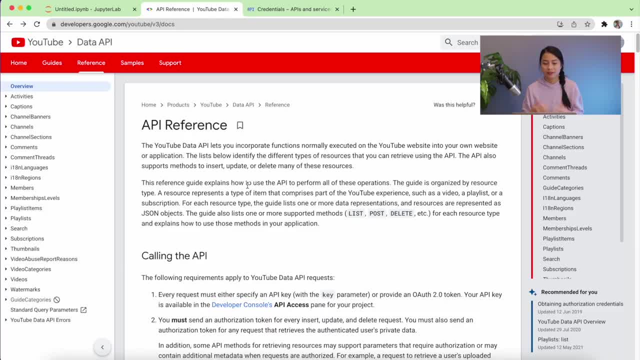 from the video ids, we can retrieve all the information of the videos. now let's go to channels. this module, basically i'm just going to install download playlist and then i'll saving everything on my site like your, either in my windows or youtube will help you out in one of these channel. playlist items so you can use any of the channel items. i think i'm saving. for some reason i'm saving from youtube. i have my docs and whatnot that have many ghost months, but because of the videos i use them for kind of the video content type: contributions toять laura-serial energy for how to get new. 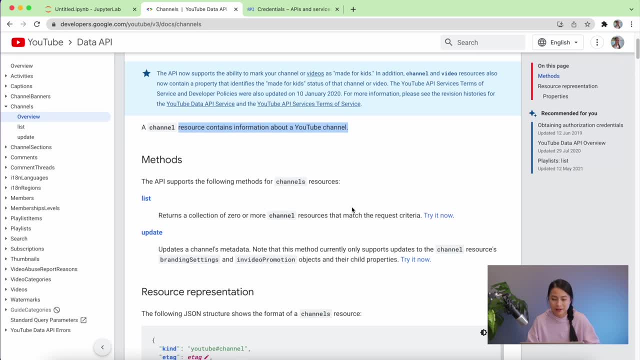 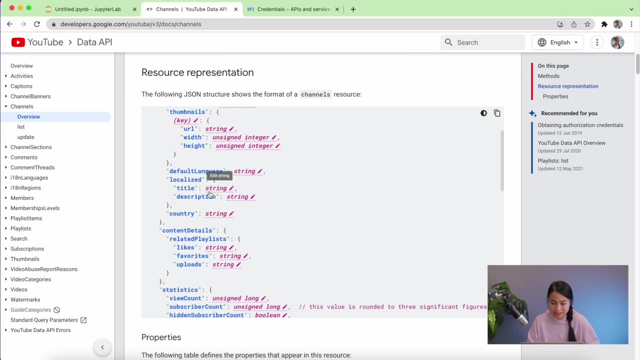 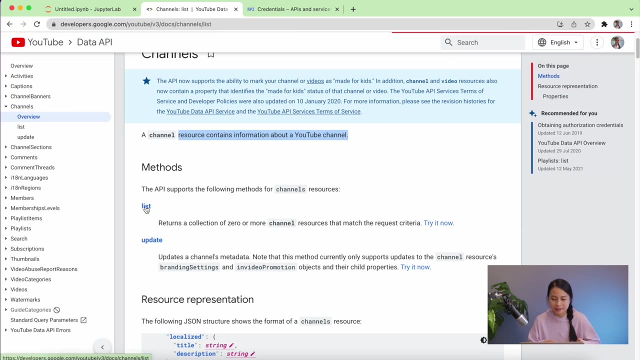 gives us information of the channel. if we scroll down here we can see all kinds of information that we can get, such as the channel name, description, upload, playlist ID, view count, subscriber count, etc. we go to the list method, then click on the icon or the code icon next to the list by channel ID over here then scroll. 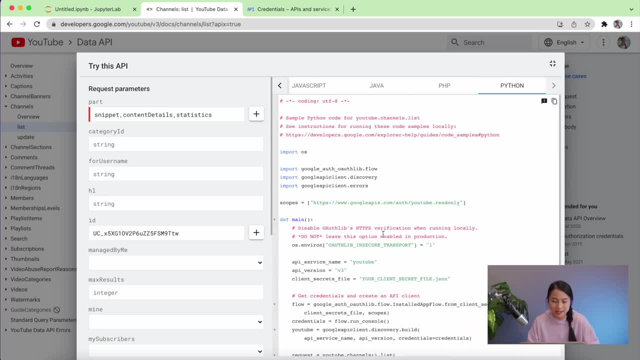 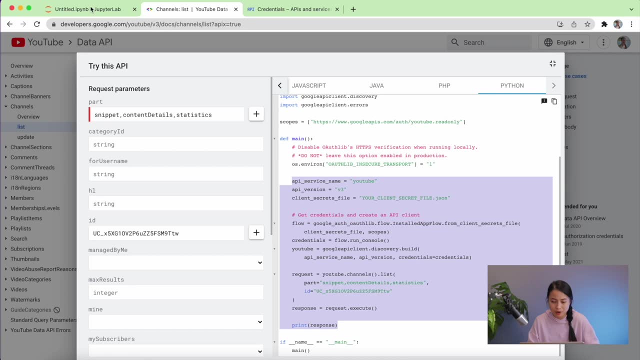 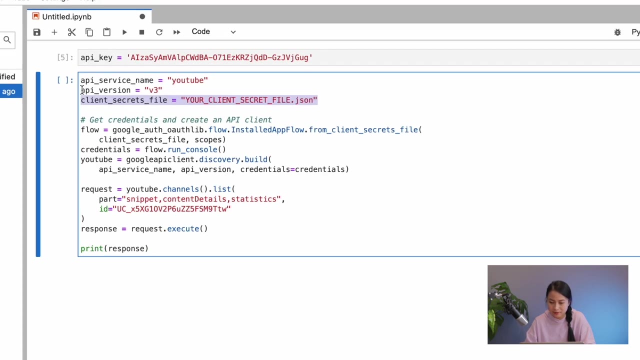 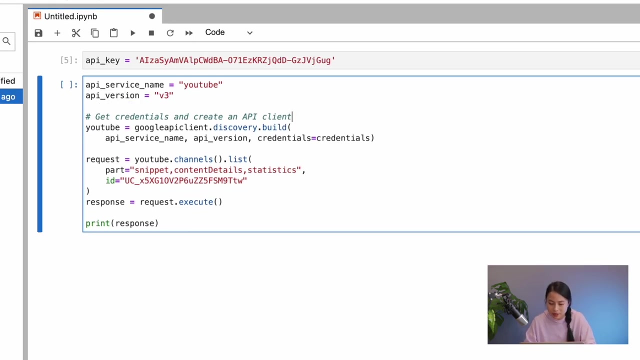 to the Python tab, because we are using Python. this is basically what we need to do. I'll just copy this whole thing into our notebook to see if we can make it work. so, first of all, we don't need this client secrets file variable, because we are not doing user authentication, but we are using developer key. so so, for this, 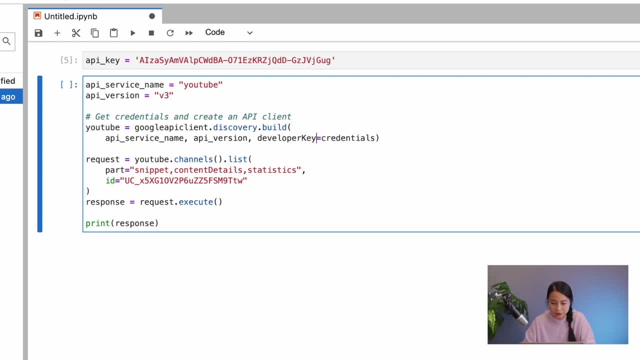 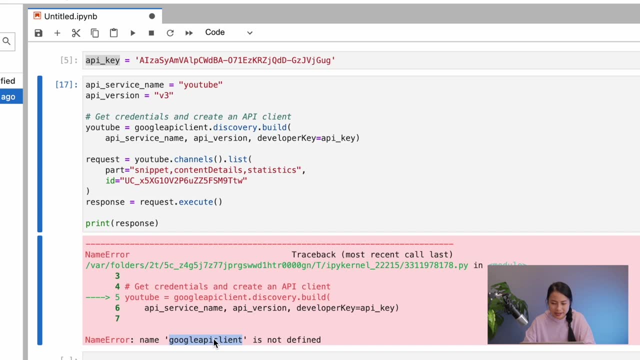 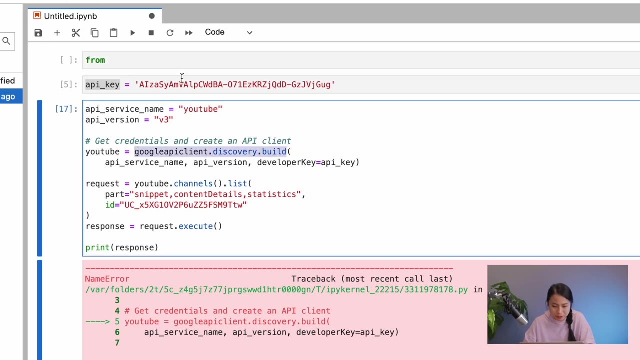 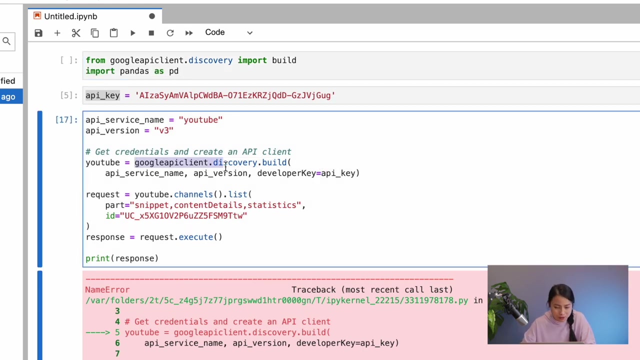 YouTube build object. here we'll replace the credentials with our developer key. okay, let's run this. we got an error because we haven't imported the Google API library, so let's import this module and also pandas as well, because we're going to need it later. now we can replace the this whole. 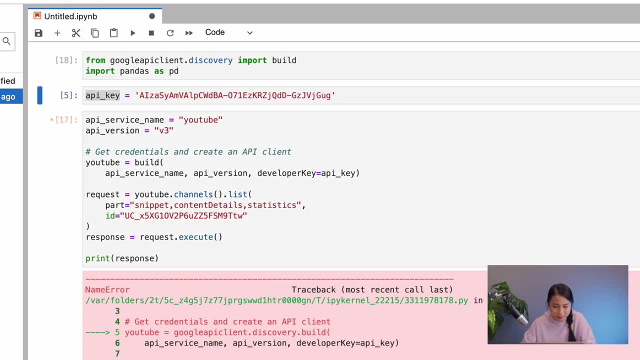 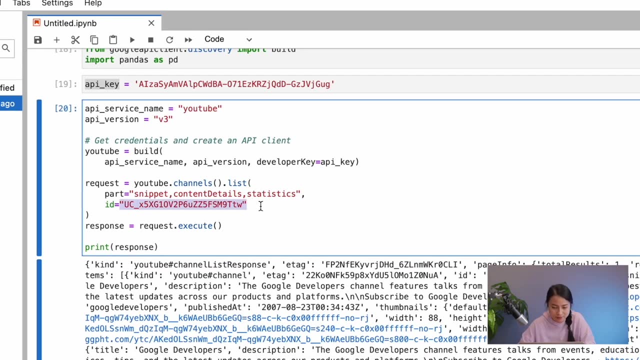 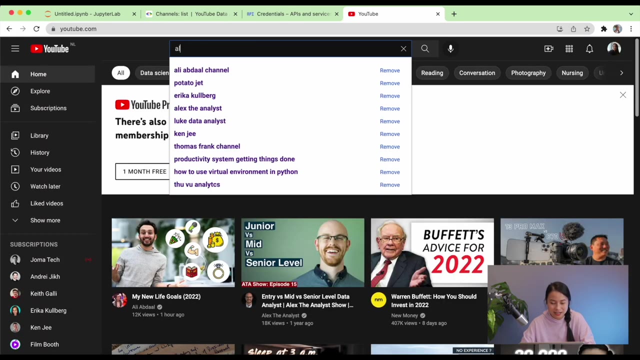 thing with the build function, because we have already imported this. now it actually works. now let's replace this channel ID with a list of the channel IDs that we are actually interested in. I want to analyze this channel. let's go to YouTube and search for this legendary man. 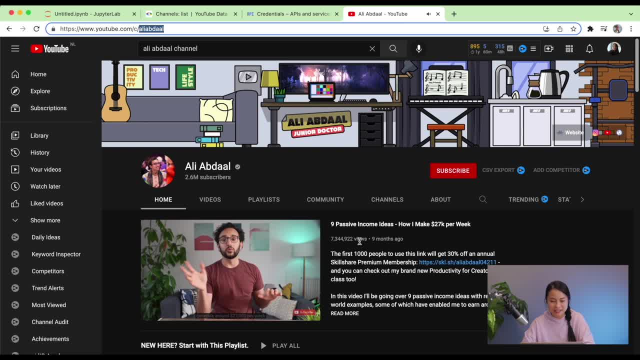 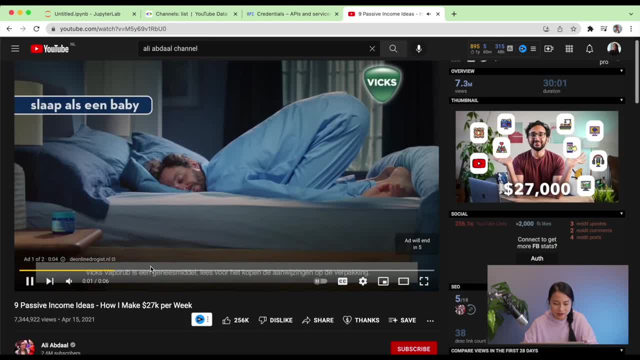 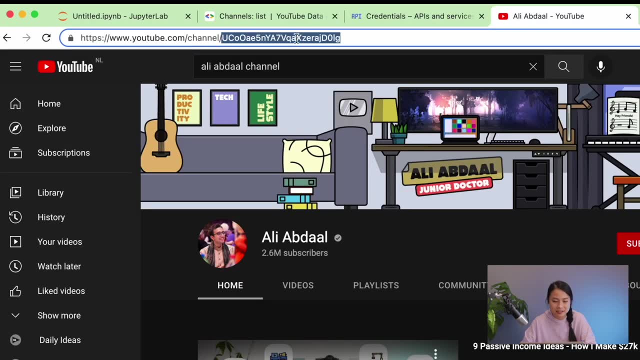 on the URL. here you don't see his channel ID. but there's a trick to find out the channel ID of any channel. let's click on any of his videos, then click on the on his profile on that video over here. so you see, now that the channel ID now appears on the URL, let's copy that. 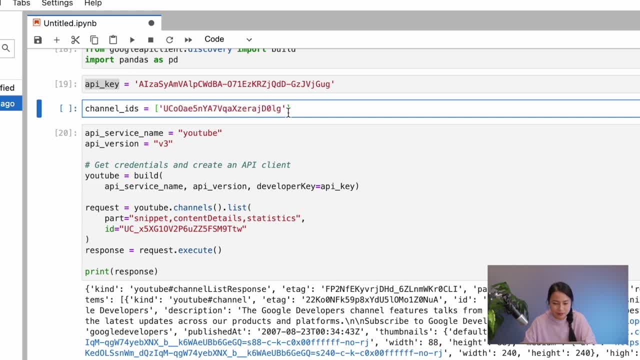 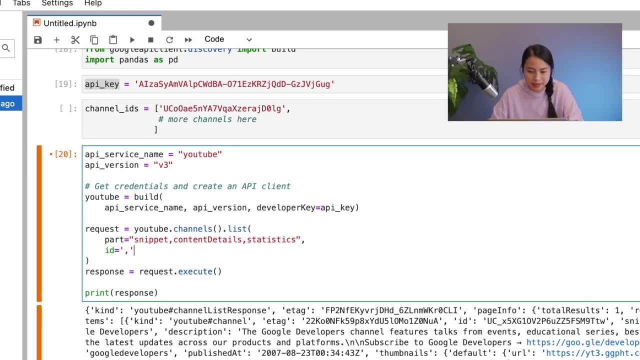 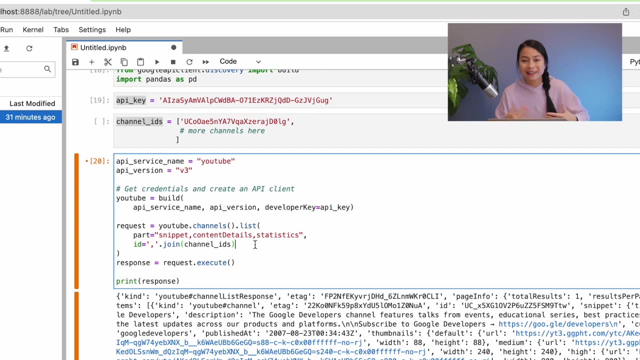 of the URL into our notebook. we then do a comma, join and channel IDs. this is to concatenate all the channel IDs together with the comma. well, in this case we only have one channel ID, but later if you want to add a lot more channel IDs to to get the data from those channels all together, then we'll need to do this. 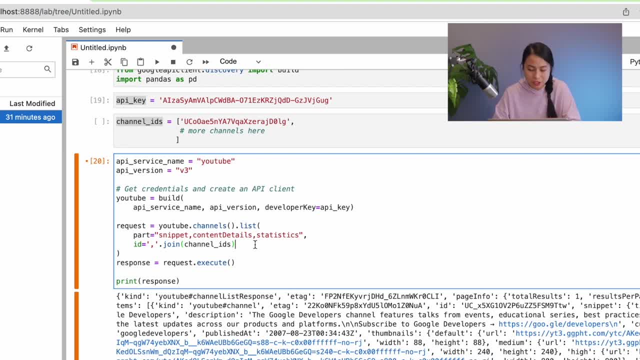 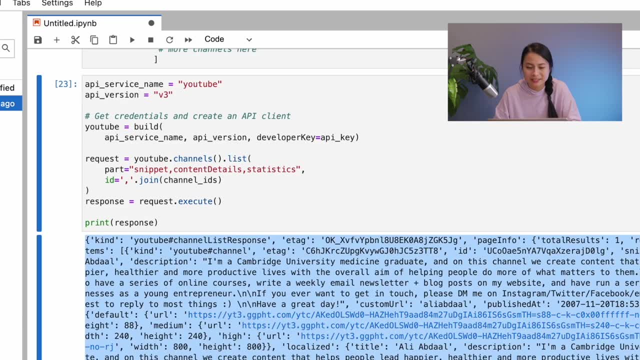 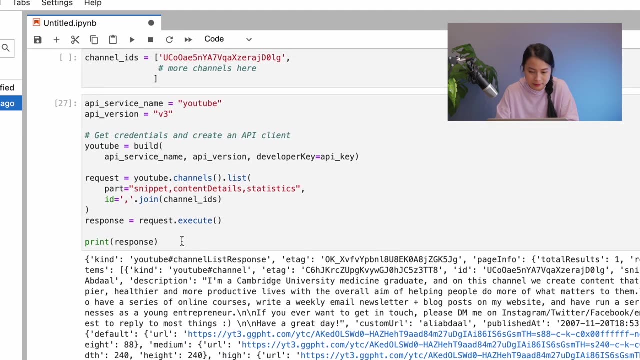 method so that it also works for multiple channels. then the response now should include the response items for all the channels in our list. let's try that, but this looks terrible. right, let's make it prettier by using the ipython display module for json. now, if we put it into the json function, it looks much nicer and easier to. 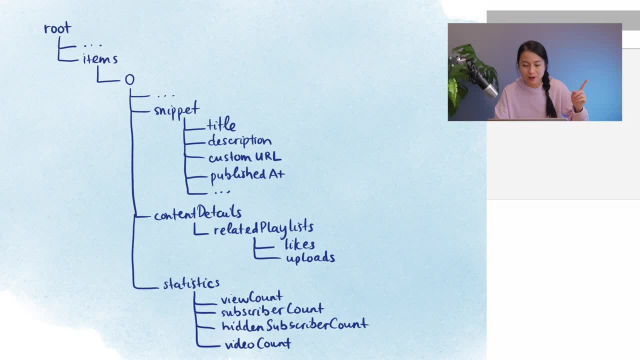 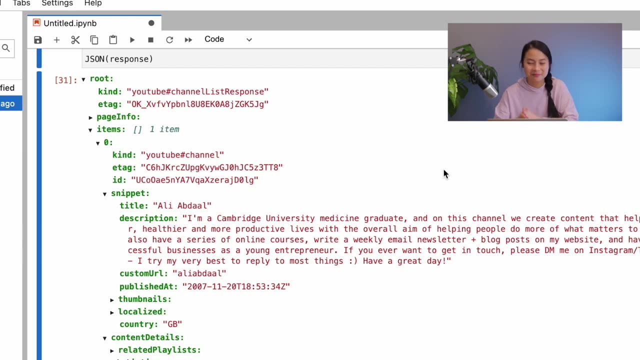 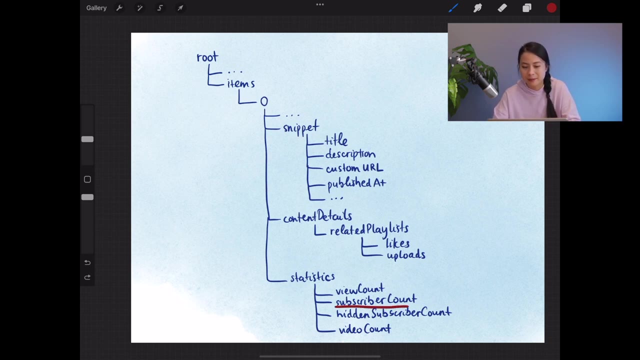 understand. i'll just quickly draw the structure of the response here to make it easier for you to to follow. this is really the hardest part of the project, but we'll get through it. please bear with me. now. there's a few interesting info we might want to extract from this response. for example, 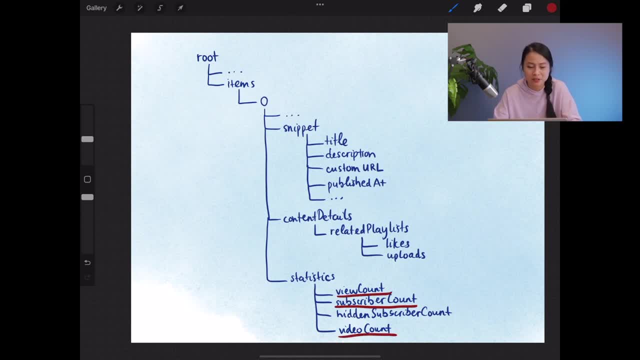 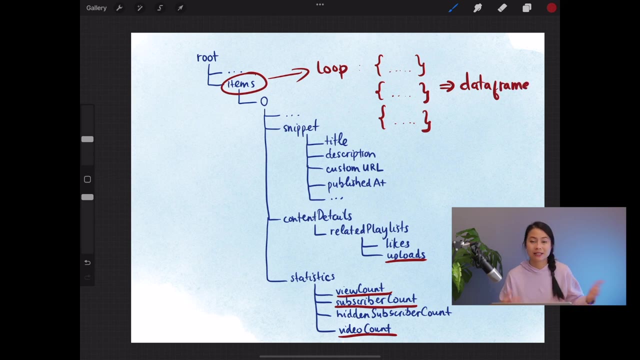 the subscribers, the views, total videos and, most importantly, the uploads playlist id. our strategy would be to look through each item in the response, extract all the information of the channel and then store it in a dictionary. so if we have 10 channels, then we'll just end up with 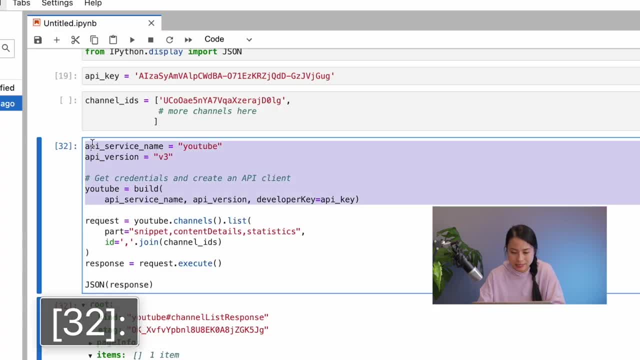 a list of all the channels that we want to extract from the response and then store it in a dictionary- 10 dictionaries. okay, then in the end we'll just need to append all these dictionaries together to make a data frame. so let me go ahead and do that. 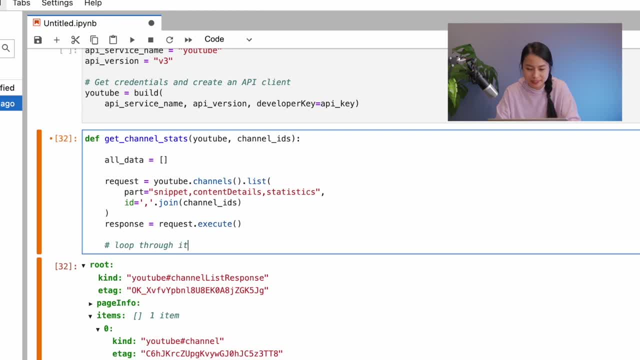 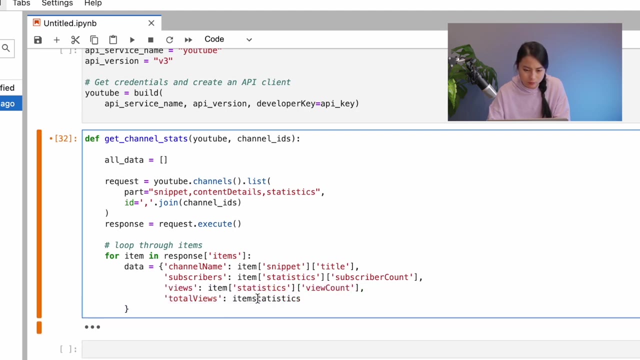 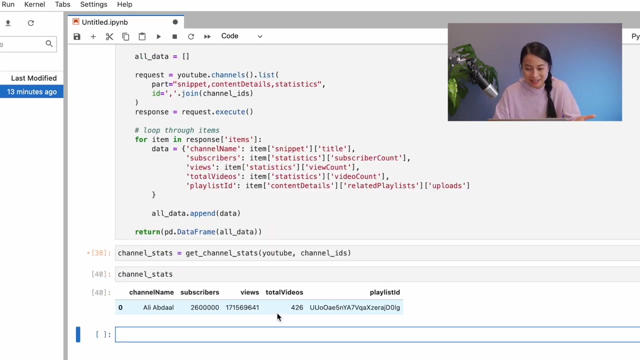 i'll create a function called get channel stats for this out, and i'll speed up the video a bit here. let's try out this function and print out the output. yeah, it seems to work and, wow, aliabdao has made 426 videos. well, i've only made 25 videos. 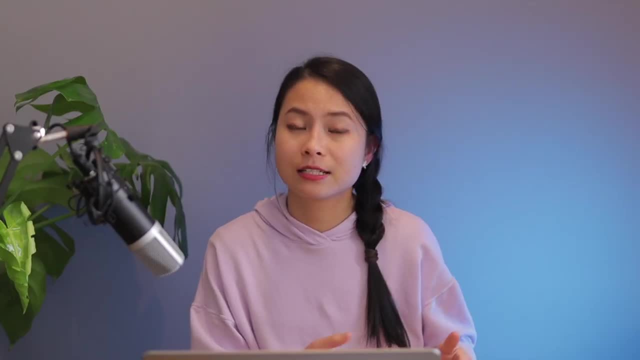 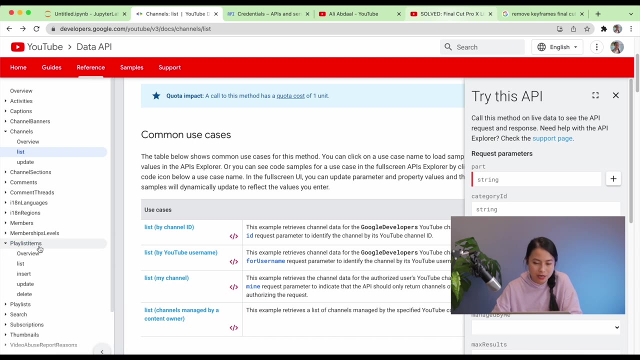 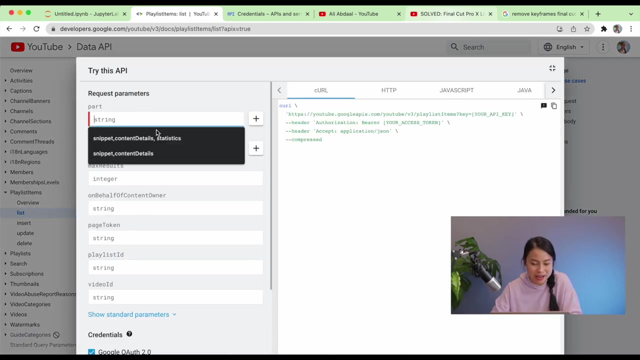 and i'm already so proud of myself. you know. the next step for us is to use the playlist id to get all the videos id from the channel. in the youtube api references we go to playlist items. this is the method we are going to use, actually very similar to what we have done just before for the channel. 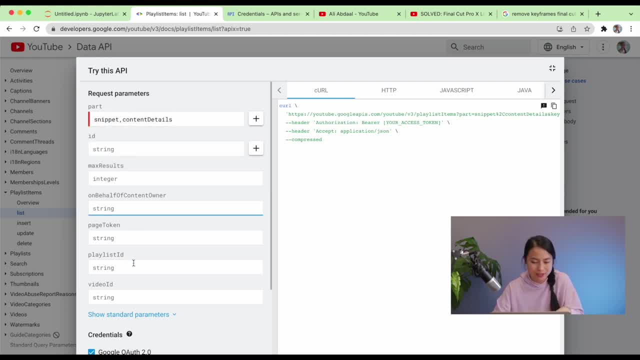 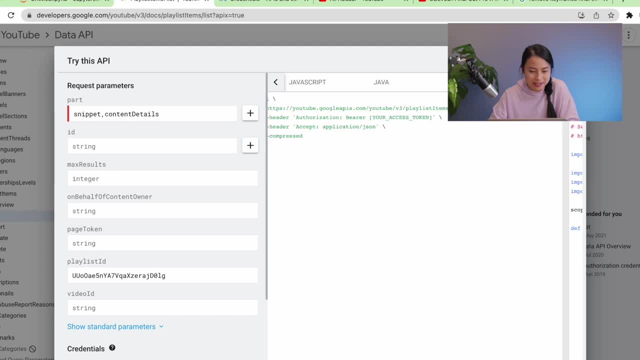 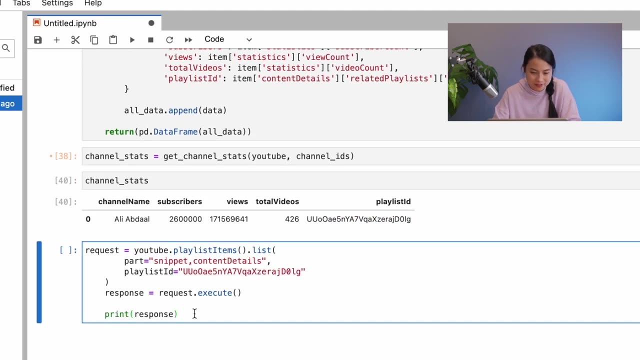 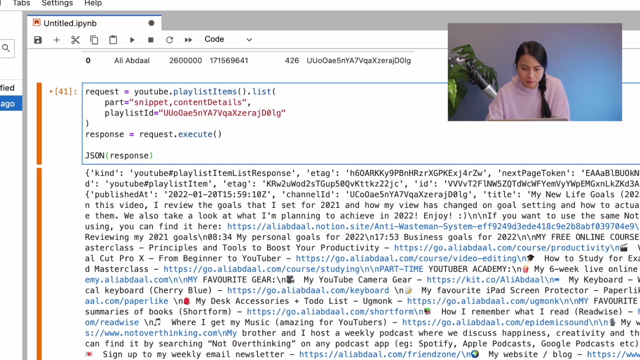 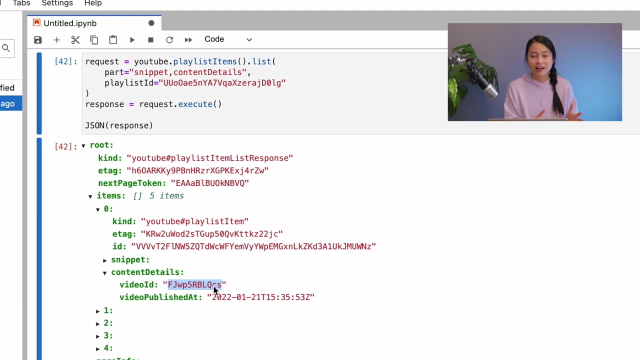 stats. we don't need statistics, because we just need to get the video ids and the playlist id of aliabdao. we just paste it here. then let's copy this piece of code into our, our notebook and then we just try to run the response. okay, that seems to work now. we'll just create an empty list to store all the video ids and then we 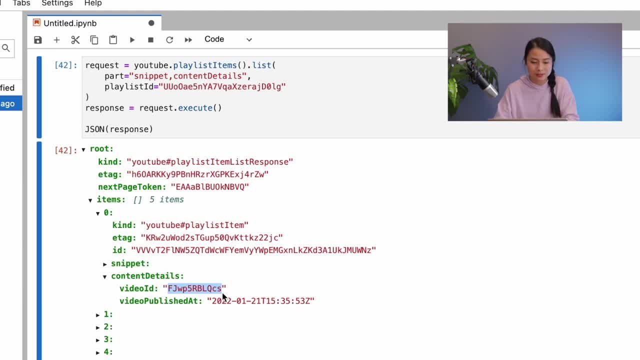 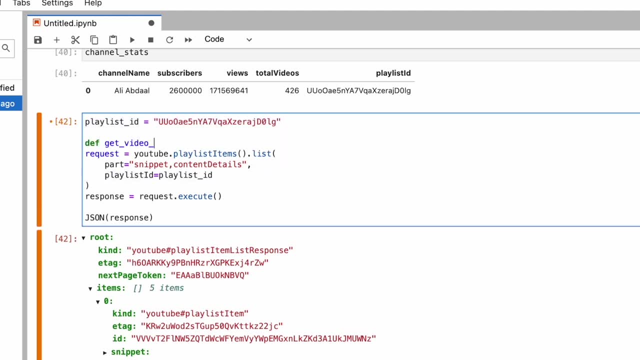 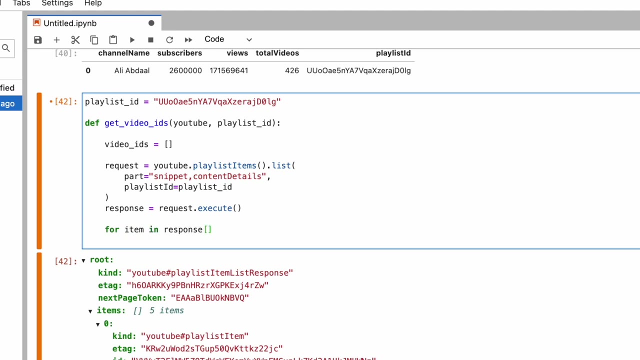 just look through all the items and append the video id into this list. let me just quickly do that. you can see all the video ids have been stored into the playlist, and then we just click the save button that we have just created. so this seems to work, but the problem is that we only get five video ids, as you can see. 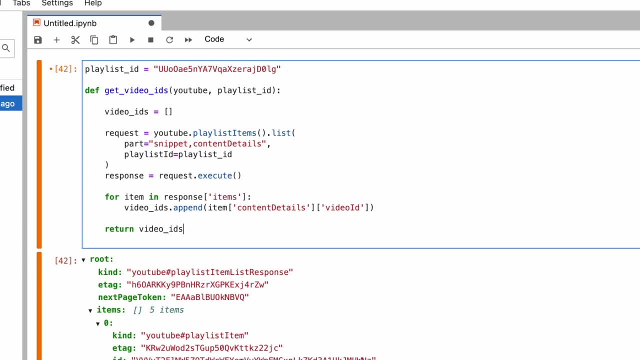 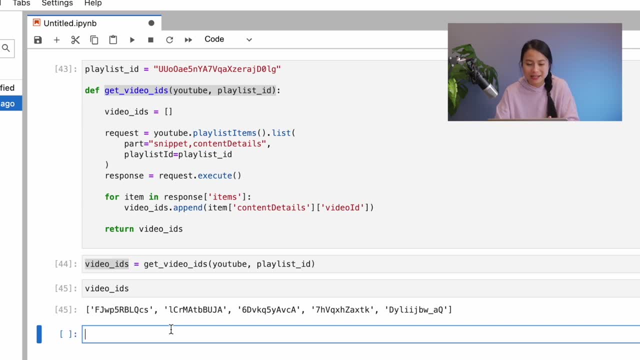 and we know that aliabdao actually has 426 videos and we don't need to add either of them. so we're going to look through the list to get that list and we'll see that this is the list that we have on our ios list and we also have a video ids that are only available in enfield. the following video is gonna be the one that is currently available on Aliabdao, and the video ids that we will be seeing today will be the video ids that our viewers have already found, and the video ids that we will be seeing today will also be the video ids that we have already found, and we will also see that movie videos and so on. 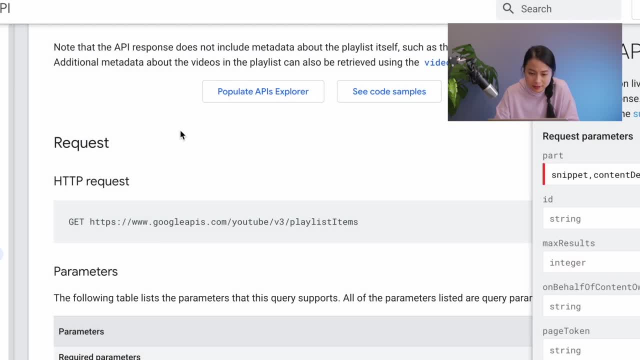 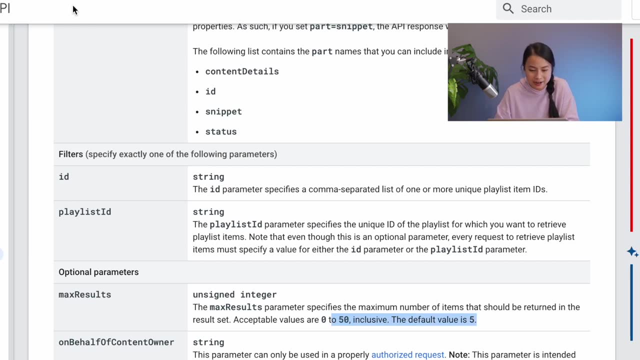 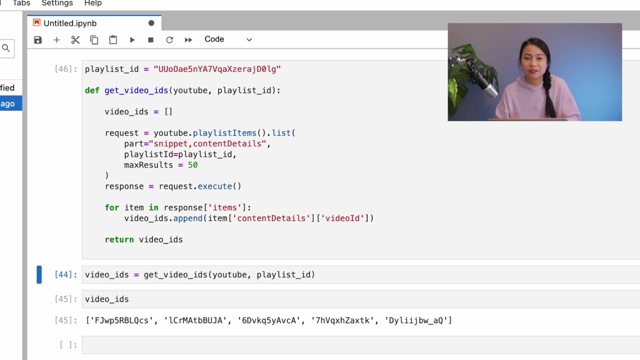 much more than that. so, from the documentation, the max results parameter is default to 5 and that's why we only get 5 items or 5 videos. now we will change it to the max value, which is 50, so we'll get 50 videos with this request. 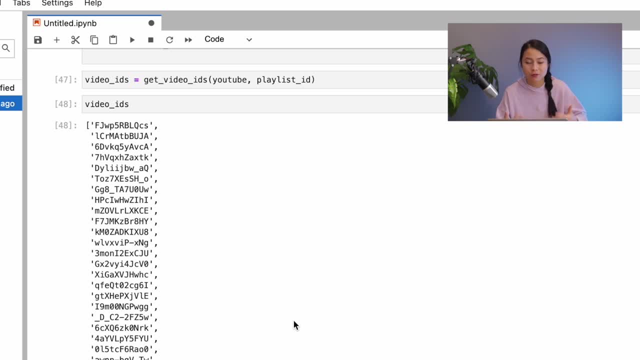 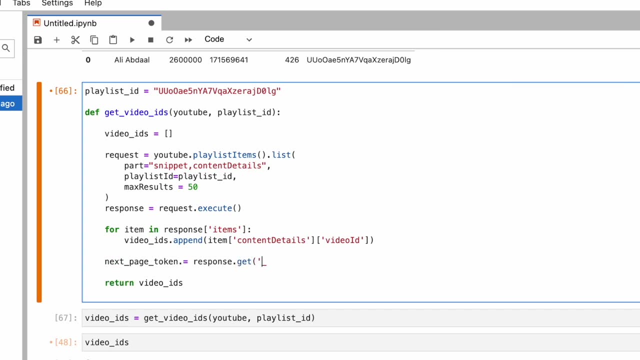 but 50 is still not enough. we want to get all the 400 videos, so we have to implement something with the next page token. so so long as the next page token is not none, we will run the request again until we reach the last page. let. 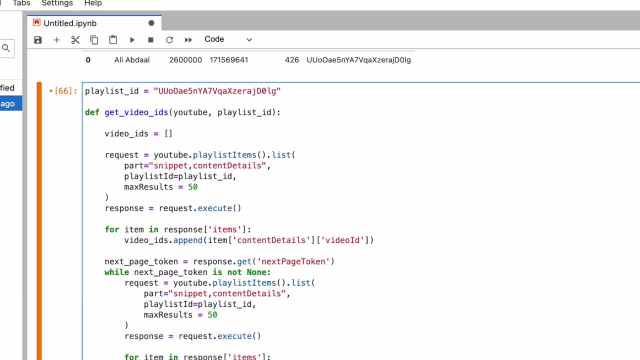 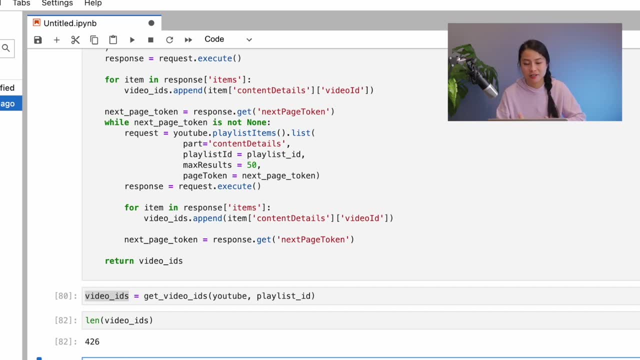 me go ahead and do that with a ugly wow loop. now let's try out this function to see if everything works. yeah, it seems to work, because now we have 426 videos. perfect, now it's time to extract the video information based on the list of video IDs. Let's take a look at the documentation again. Go to videos. 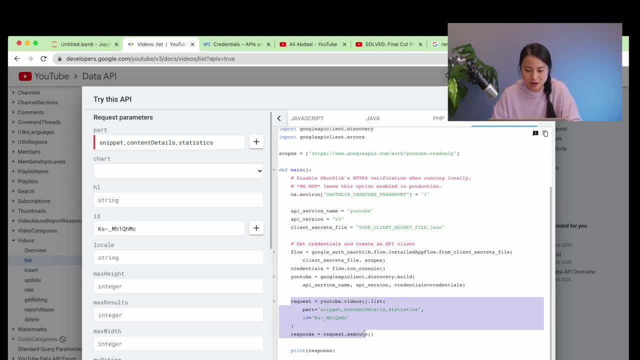 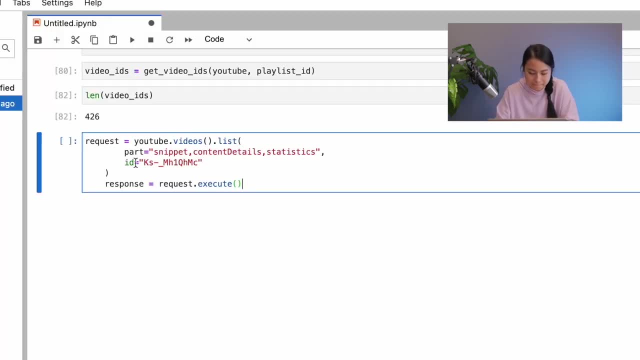 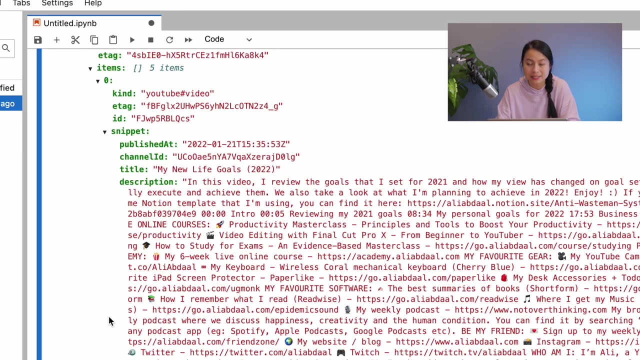 and the list method. Then we'll just copy the code here to our notebook. Let's try this for the first five videos and print out the response. There are quite some interesting stuff here, So I'll make a dictionary of all the things that I want to extract and then create an empty dictionary to store all the video info. 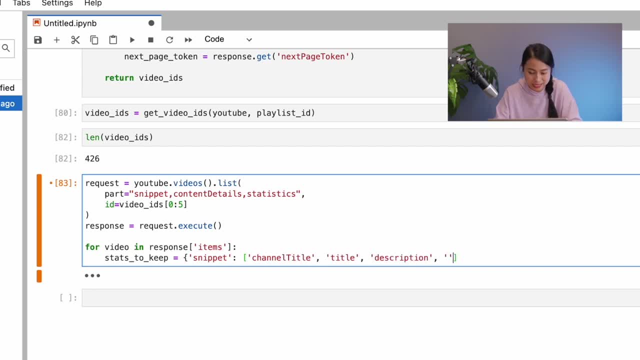 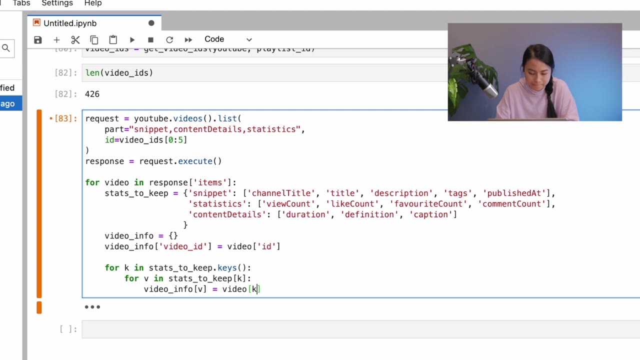 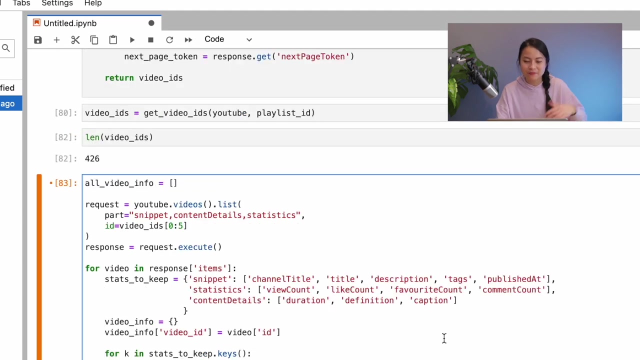 So for each key value pair in this start to keep dictionary, I'll extract the video information from the response and then save it to the video info. Okay, Okay, I've done this before, so I know that something will go wrong. It is because some videos will. 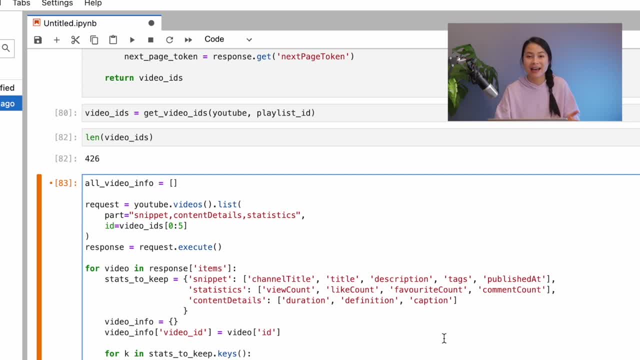 miss certain information. For example, some videos don't have any tags. Probably Ali just forgot to put the tags in So to prevent getting this kind of error. we'll implement the try except here, So uh, so if we get an error, we'll assign the value to none. Let me finish. 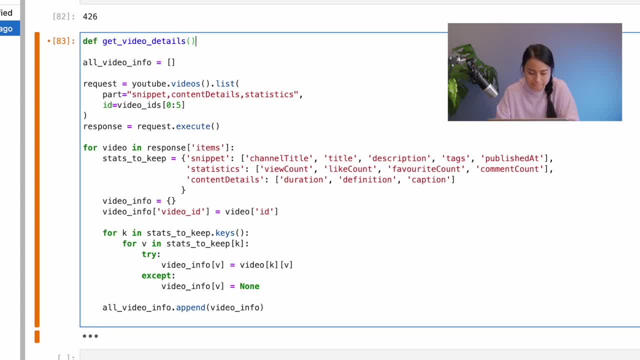 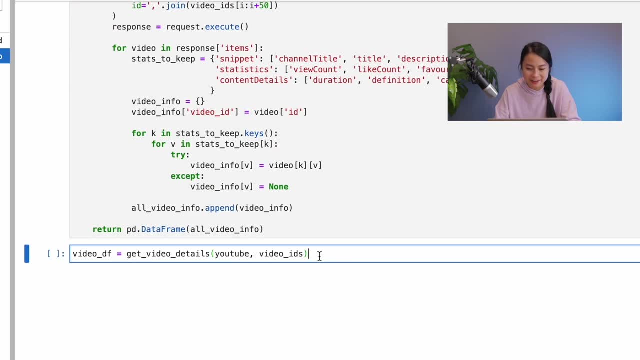 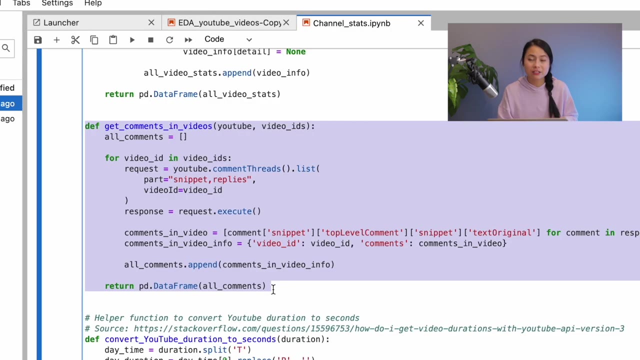 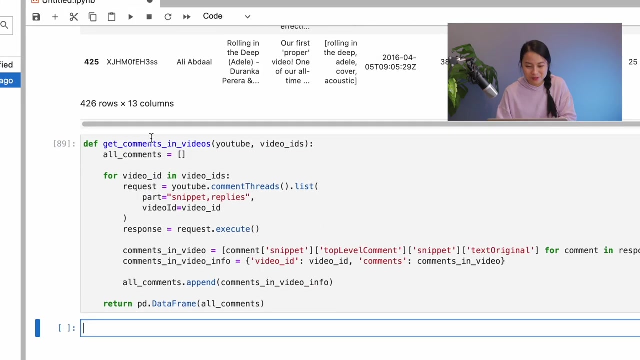 up this get video details function. Now let's try it out. And yeah, luckily it works. And this is the final data set from all our hard work. I also made a bonus function here for you guys that also extracts the comments from the videos. I find it really funny to read through all the comments people made. 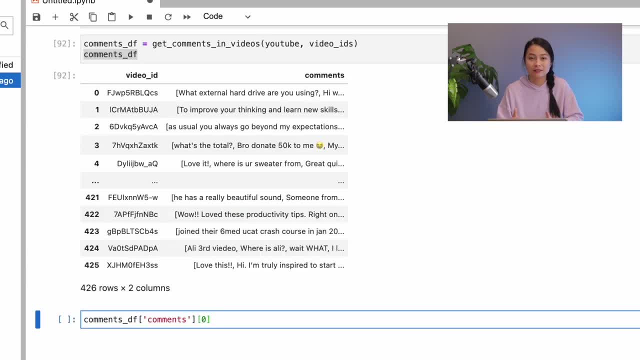 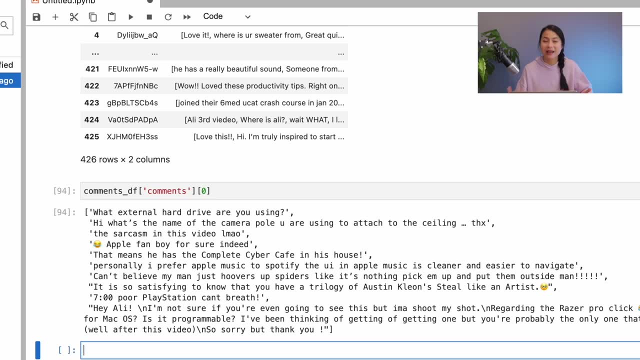 And, more importantly, we can do tons of analysis on this huge amount of text. I'll link the final code to this project in the description down below so you can check it out and run it yourself. Now that we have the final code, let's go ahead and run it ourselves. Let's. 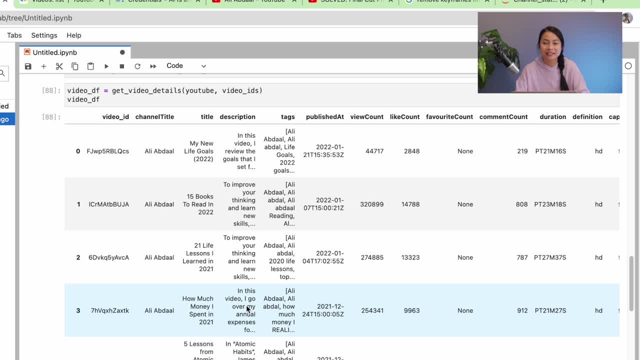 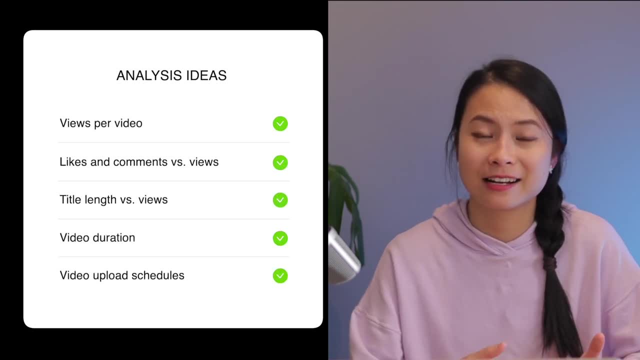 go ahead and run it ourselves. So if you have an amazing data set to work with, there are actually a lot of ways to analyze it, depending on your interests. What is the average views per video, And does the number of likes and comments really matter for views, Or does the title length also matter? 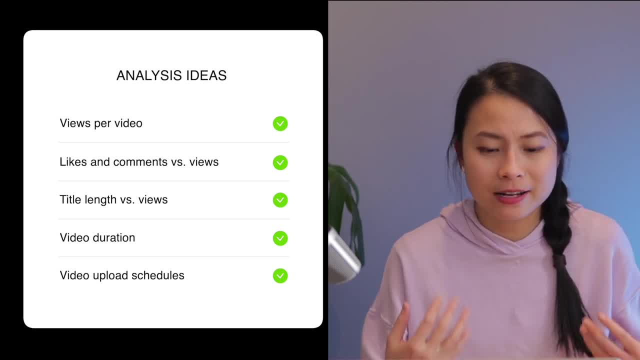 for views And how long usually are his videos And how many tags do his videos have And which tags associate with most views, for example, And how often does he upload his videos On which days in the week We can actually get all this information from. 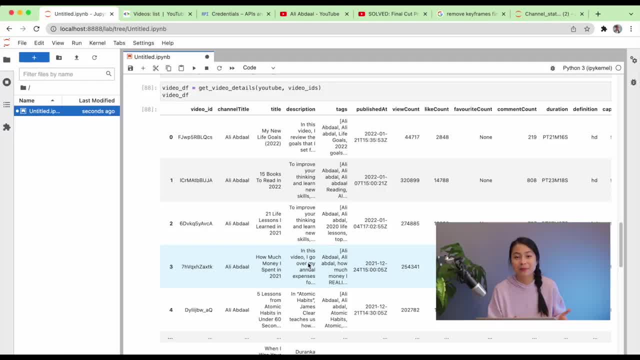 Zoom. So let's go ahead and run it ourselves. Let's go ahead and run it ourselves. Let's do a test run and see if there are any changes to the script. Let's see how many new texts we see. Let's go ahead and do it. 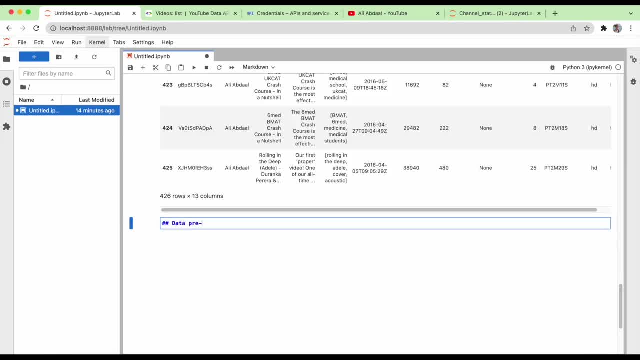 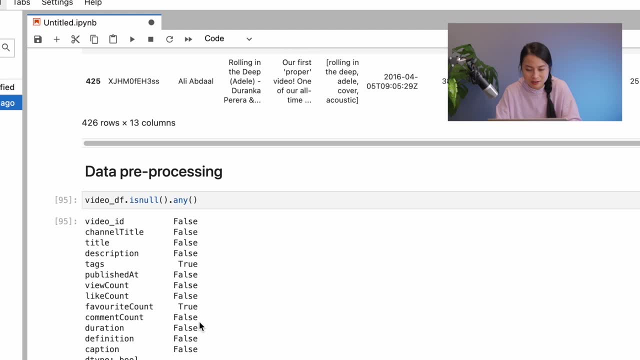 First of all, we have to do some data preprocessing and also probably some feature engineering to enrich our data set. Firstly, let's take a look at the new values. We can see that we don't really have the new values of all the columns except for the texts column. 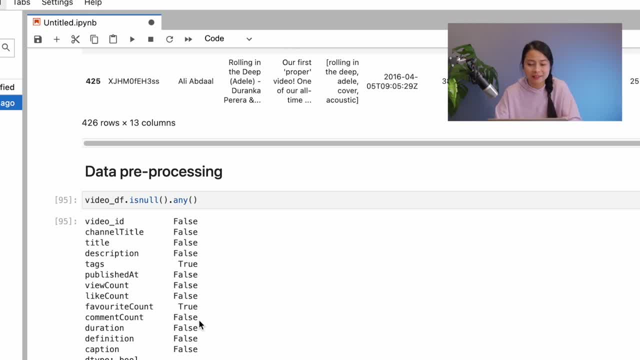 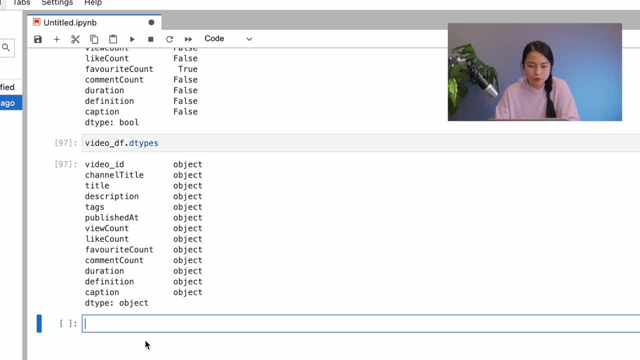 But it's not super important, So let's ignore it for now. Secondly, let's check the data types. We're going to see that all columns are in object format at the moment, which doesn't make sense for some columns like view counts and light counts. so I'll go ahead. 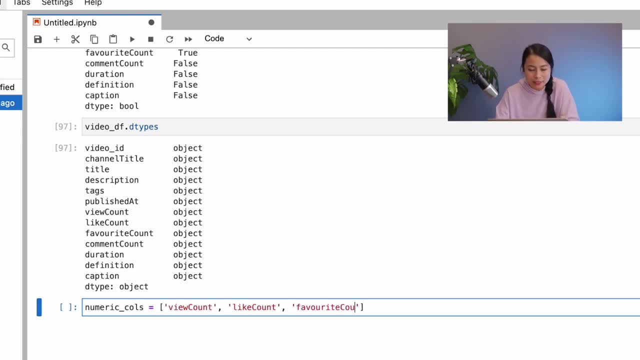 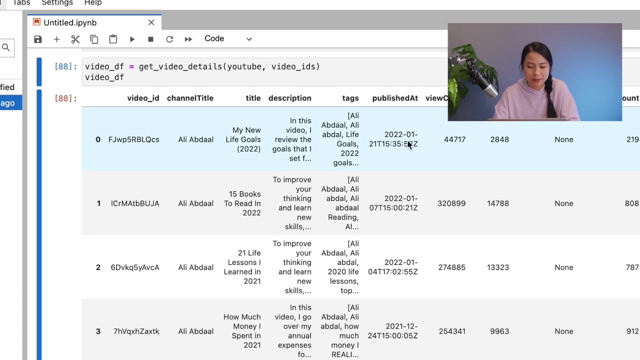 and convert them to numeric or integer, if you will. You can also do a for loop here, but in order to do it faster and in a cleaner way, I would recommend you to use an apply function here. Next, let's create a column for which day in the week he published his videos based on the 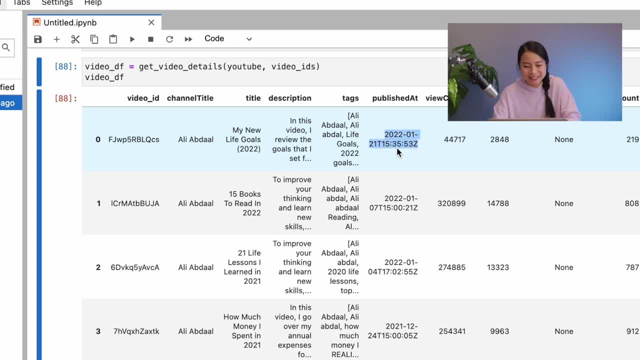 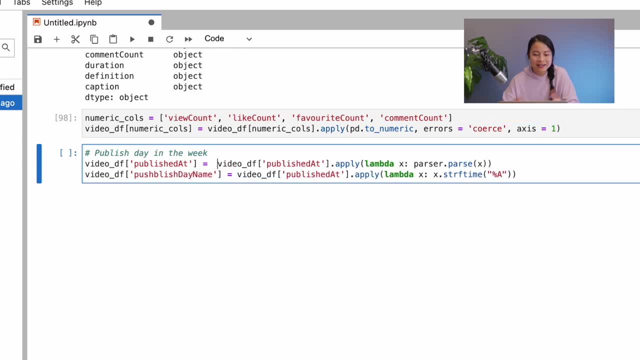 published ad column that we see here. I'm super bad with dates, so I just found this code from somewhere on the internet, so I just chuck it in. Next, we will need to convert the duration column to numeric. At the moment it looks pretty weird because it's like a 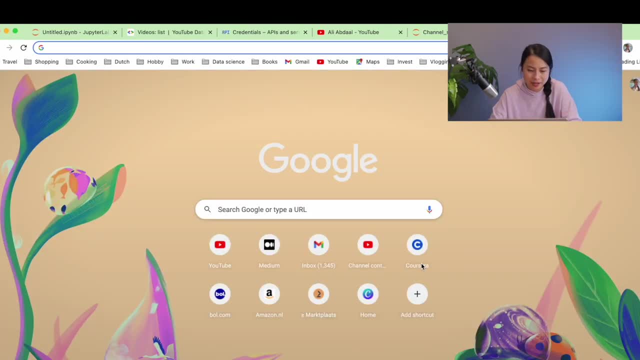 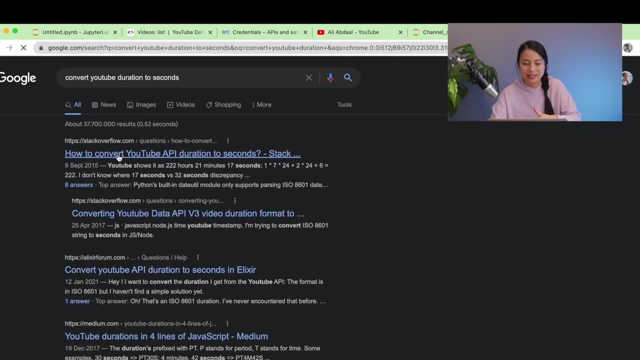 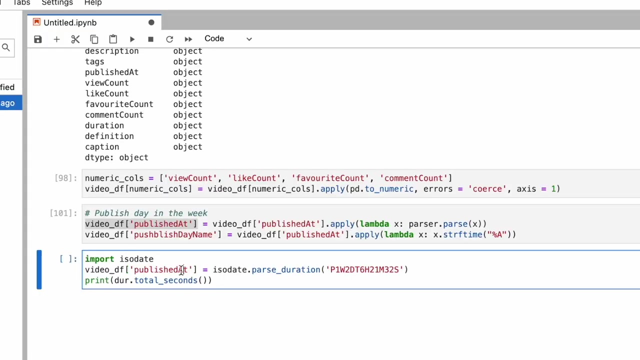 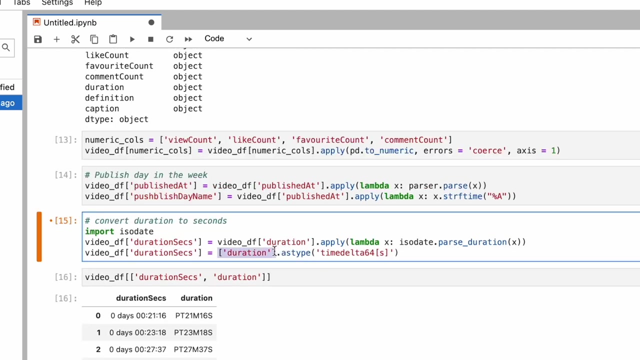 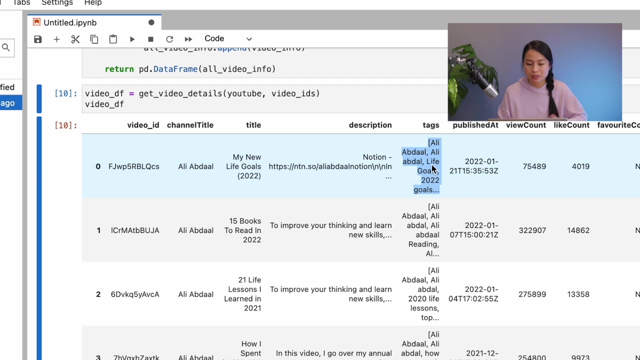 string with letters and numbers. I found on a Stack Overflow thread that talks about how to convert the YouTube duration to number of seconds, so I just copied this code here and adapted a little bit and used it. Problem solved. Then we'll add the number of tags for the video, because we also want to analyze it. 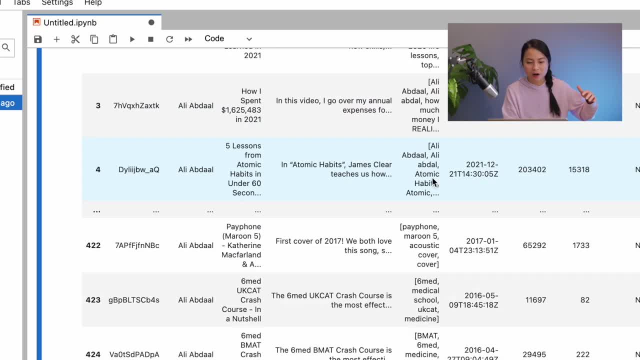 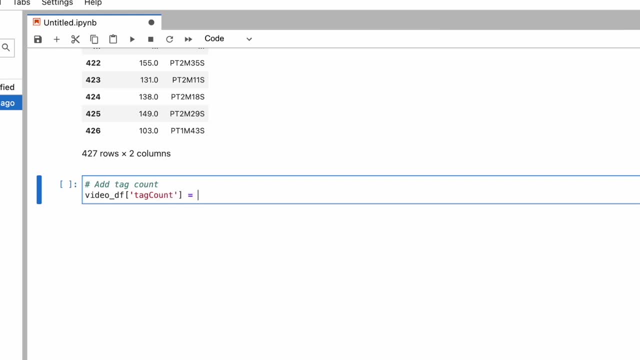 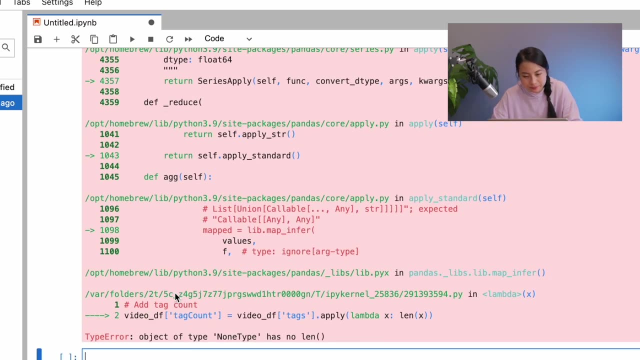 later as well. So, from the list of tags that we see on each row, we'll apply a lambda function on it to get the length of the list, which is basically the number of tags. Ah, we got an error here, because- yeah, because we- we have some empty tags in here, So we're going to 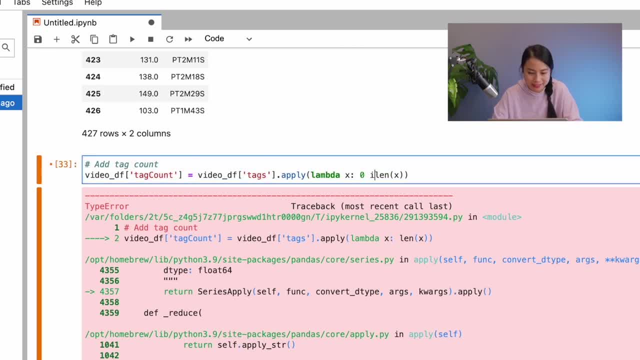 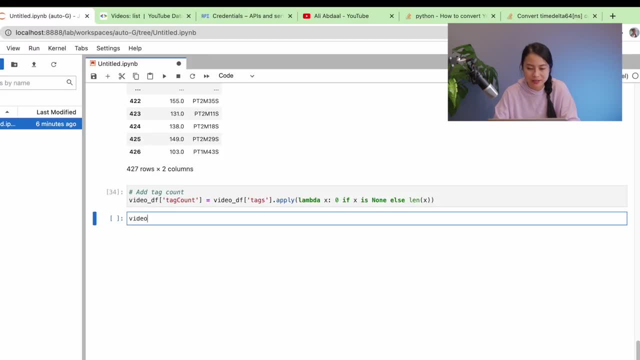 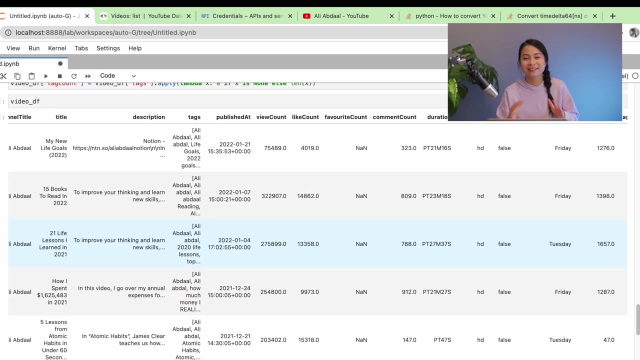 make a little if-else like this, so that when the tags is none, we will assign zero to it. Now let's print out the data set to see if everything works. That looks pretty good right Now. let's move on to the most fun part, which is data analysis. First of all, let's see what Ali's 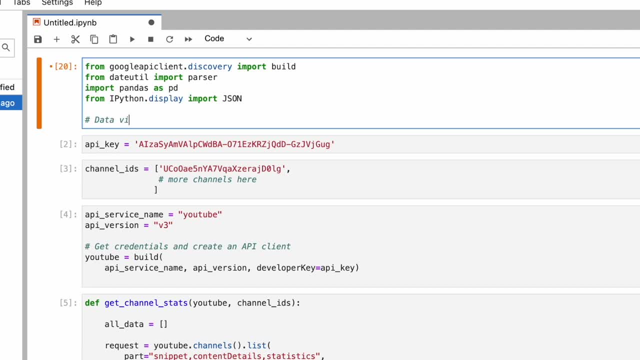 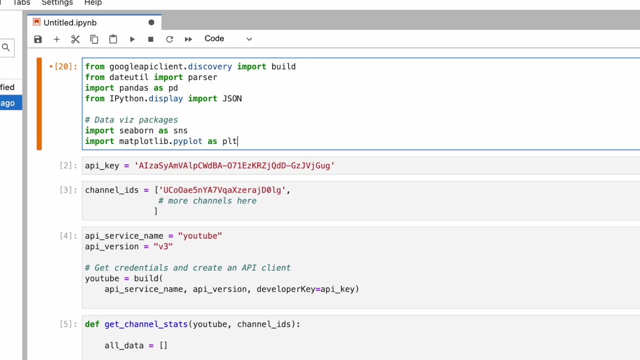 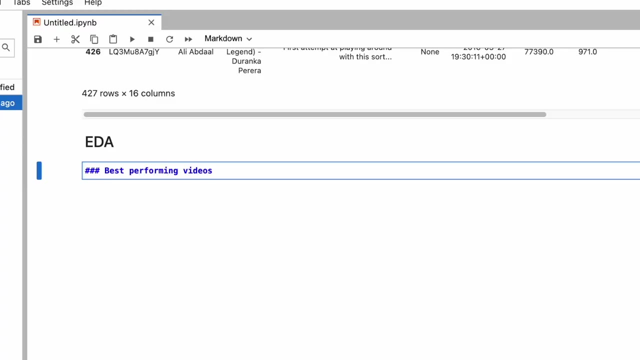 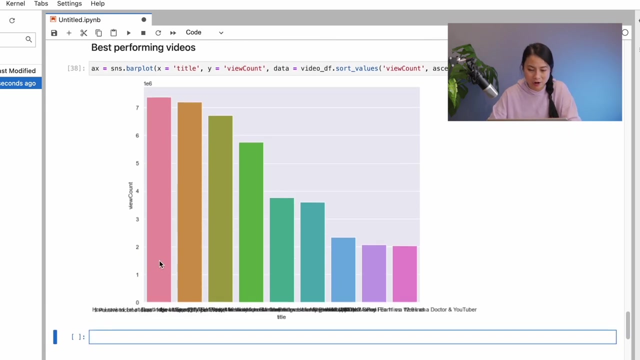 best and worst performing videos? I'm very curious. Let's import Seaborn and Matplotlib packages. Now we can make a bar chart for the view count, sorting the videos from the highest views to the lowest views. The x-axis is now overlapping because of some long titles, so I just rotate the x-axis 90 degrees. 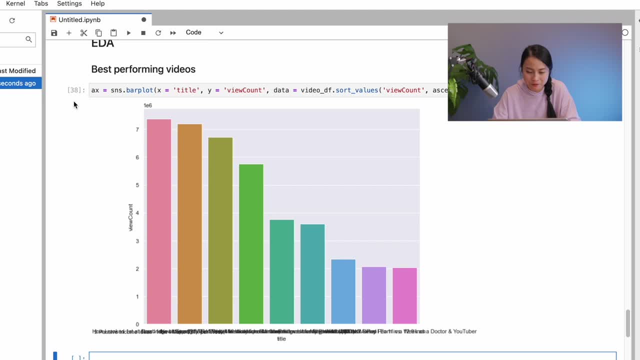 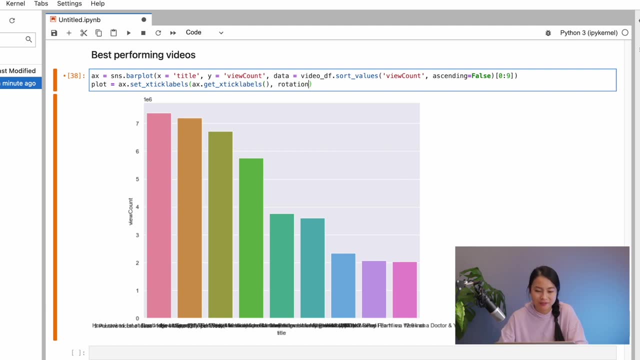 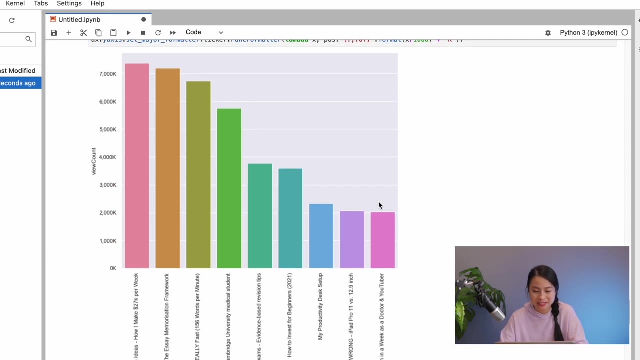 and the y-axis also has a weird number format, so I just reformat it as well. Honestly, I just googled everything and find the solution to these issues. I don't know it by heart, to be honest. Now let's also take a look at the worst performing videos on this channel as well. 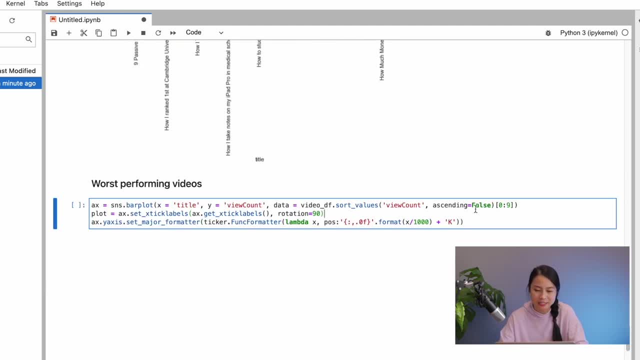 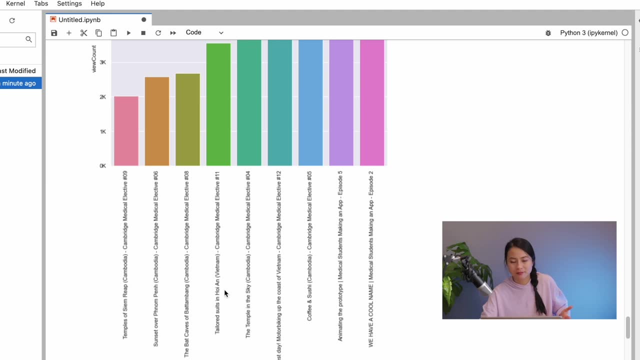 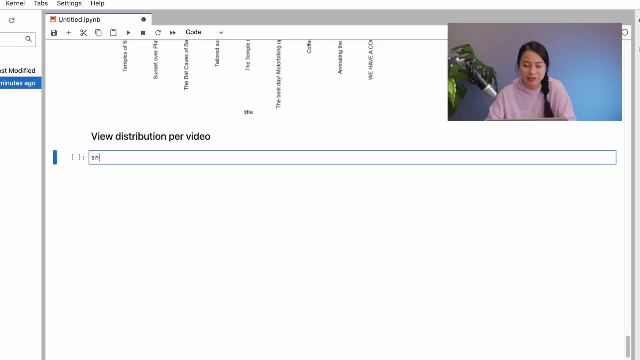 using the same function but with the opposite ordering. So from the lowest views to the highest views. Well, it seems like these videos are all his very old vlogs, I think before he became popular. Now let's also take a look at the view distribution across all the videos on his channel. 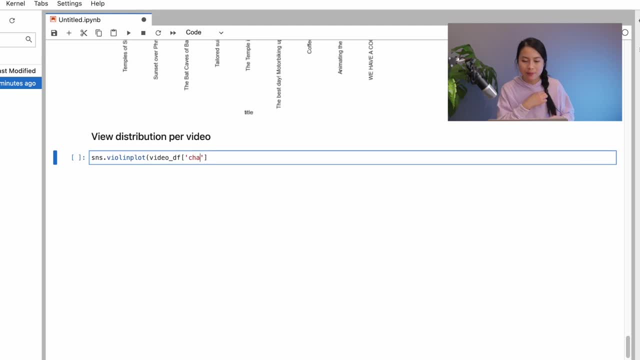 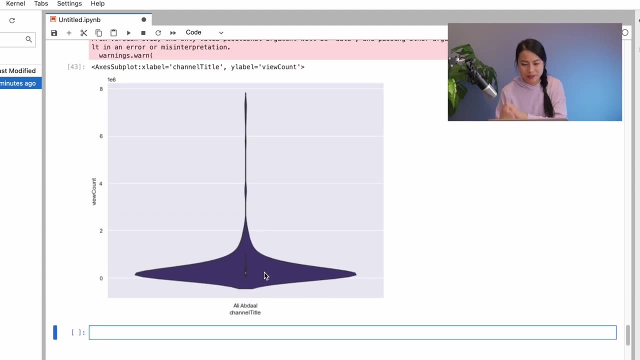 We can use histogram and the histogram will be the same as the histogram of the video distribution. different plots for this, but I'll be using the violin plot. So indeed, some of his videos are really outliers here with so many million views, but most of his videos 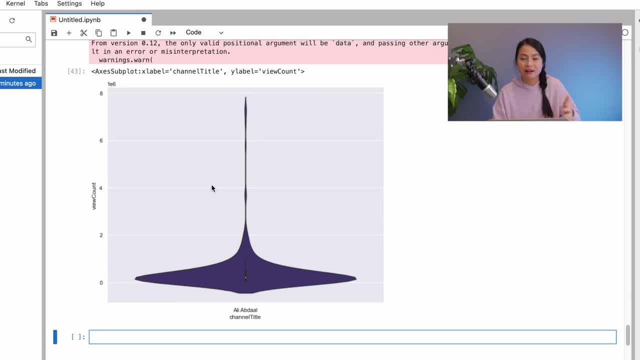 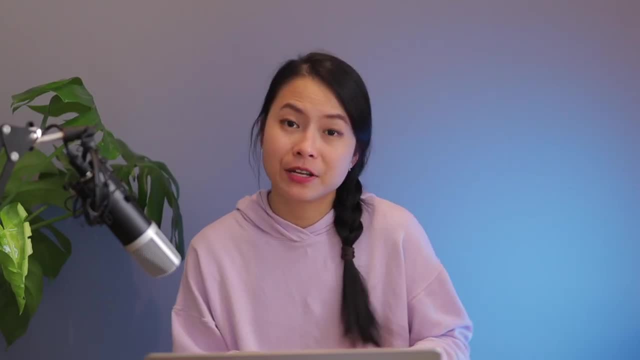 are actually just around 200 000 views. Violin plot is actually very useful if you want to compare several channels together. Next we'll plot the number of views against number of likes and comments, just to see if there's any relationship here. 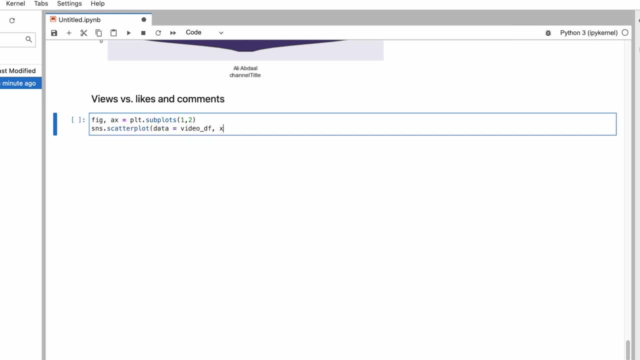 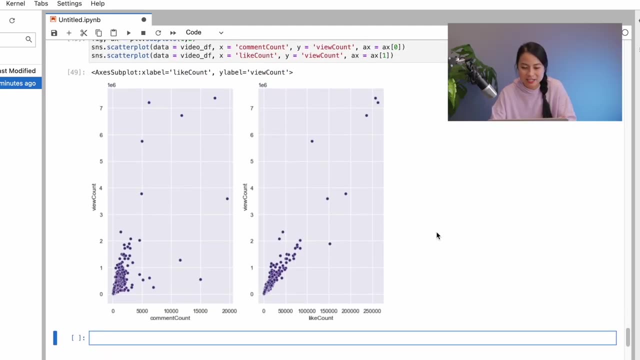 Let's do some scatter plots. It's always fun. We can see some positive correlation here, especially for the number of likes. It makes sense because the more people who watch the videos, the more likes the video could potentially get, And also the other way around as well. 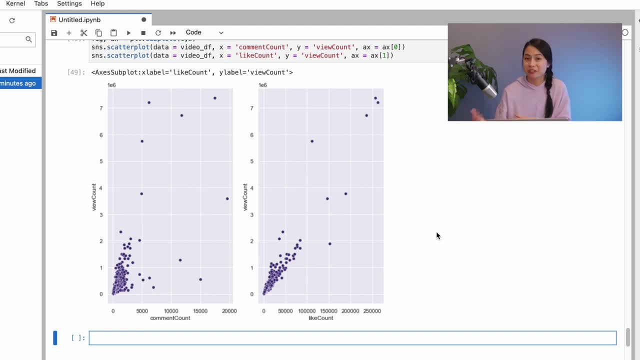 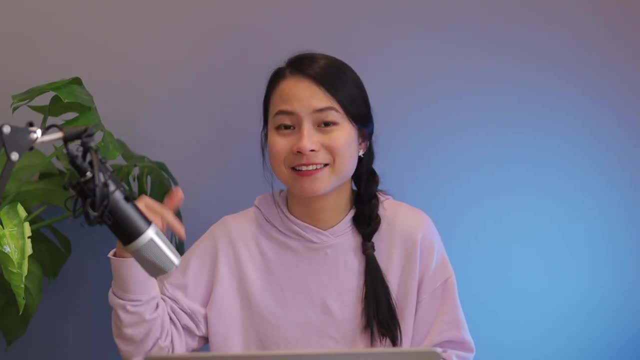 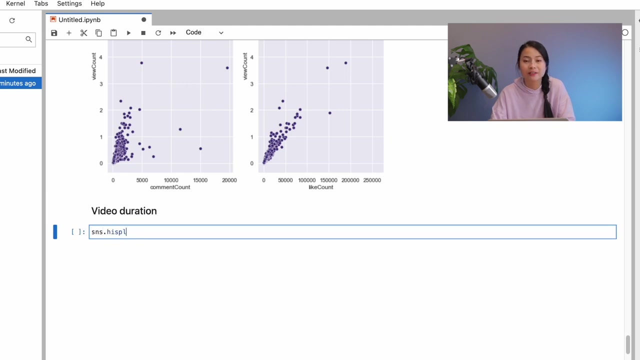 because the more likes a video gets, the more likely the YouTube algorithm will recommend it. So, based on this, if you want to support this channel, please hit the like button below to help this video reach more people. Now let's also see what's the average duration of his video with a histogram. 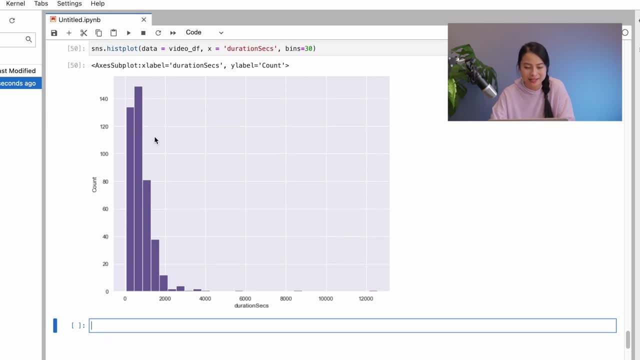 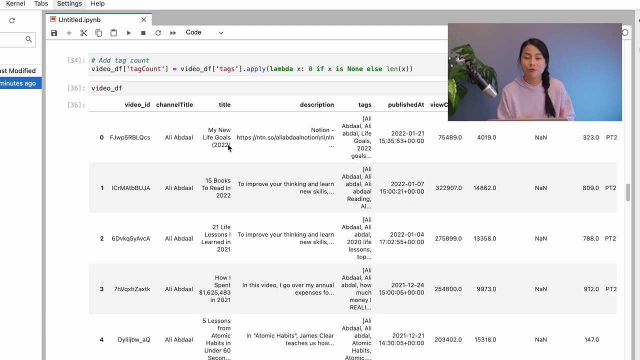 I think most of his videos are around 10 to 15 minutes. The longest video is three hours or so. Quite interesting. From the video titles we can also create a word class. Let's see which words occur most often in his video titles. 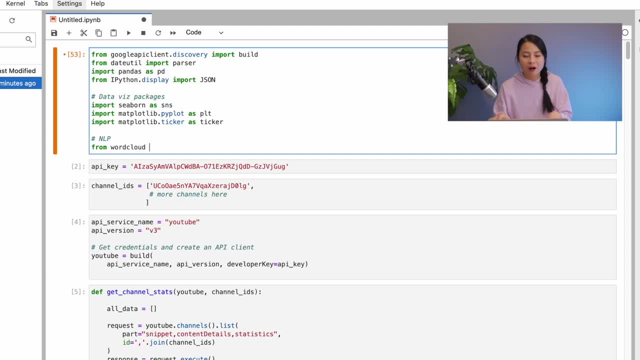 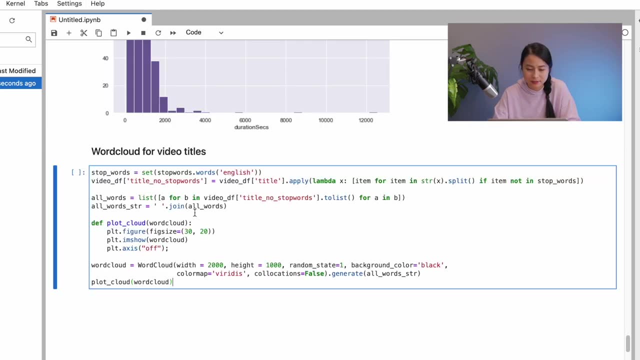 There's a Python package for this, called word cloud. I'll probably explain some more NLP concepts in another video. For now, let's take a look at the word cloud. Well, this looks so alley up. now We see, the most common words here are Cambridge. 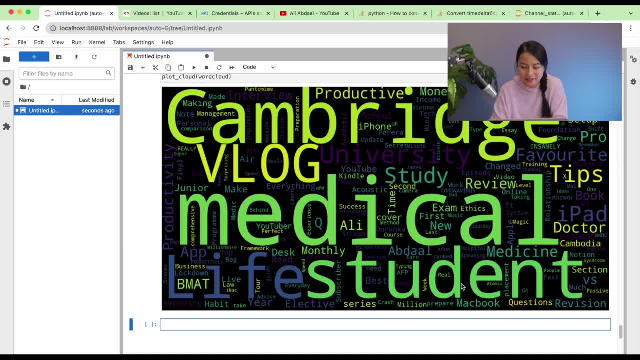 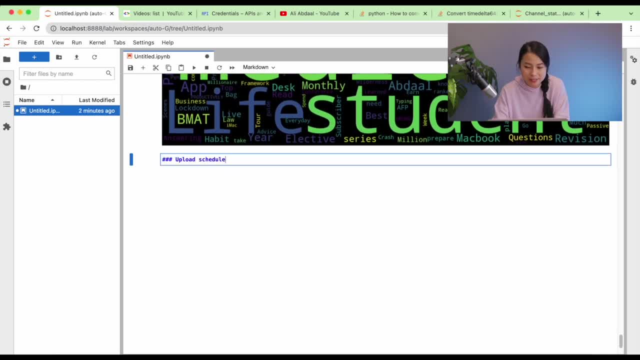 medical student life vlog and study. The last thing that I want to see is which days in the week he usually uploads his video. We can easily make a bar chart for this, But be aware that we'll have to order the weekdays manually, because 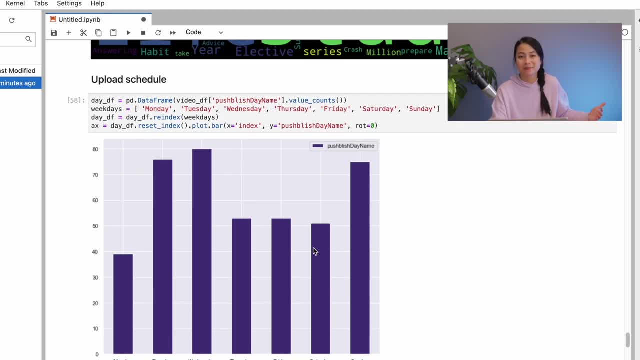 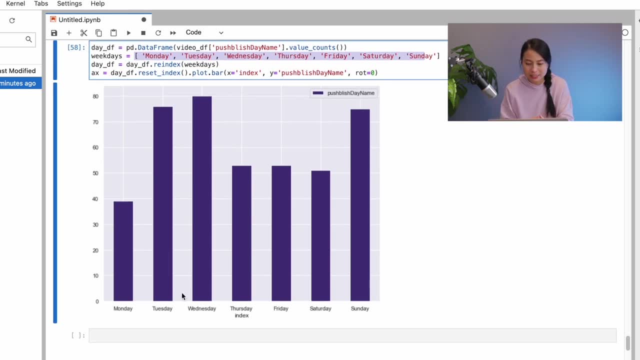 Python doesn't know which days come first. That's unexpectedly stupid, right? So I just copy what I did here. And we can see in this bar chart that he actually uploads his videos mostly three times a week, and on Monday, Wednesday and Sunday. 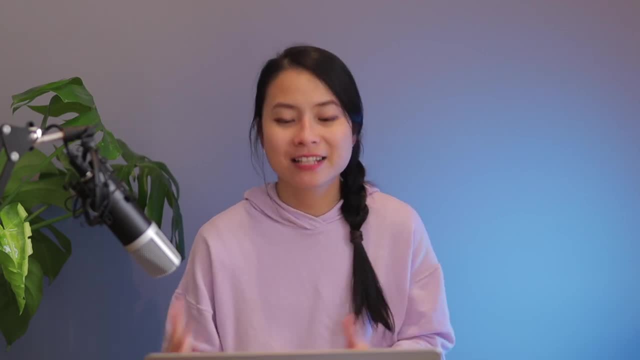 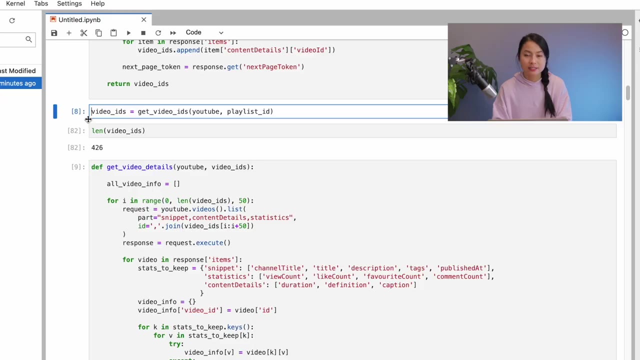 Now that we have done quite some analysis already, the final touch to our project, before we share it with other people or upload it to GitHub, is to clean up the notebook. So let's remove everything that is redundant and also comment your code. That is also really important. 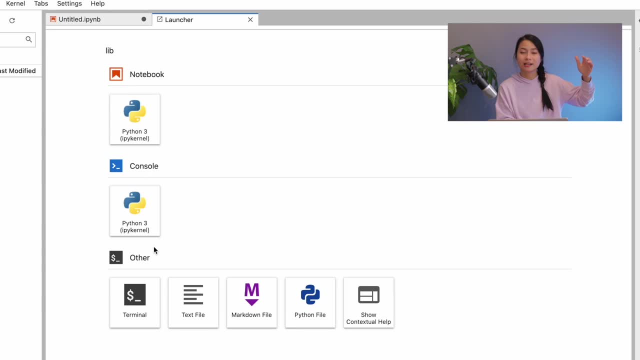 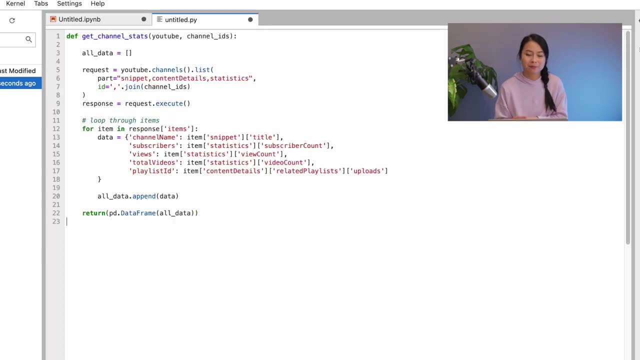 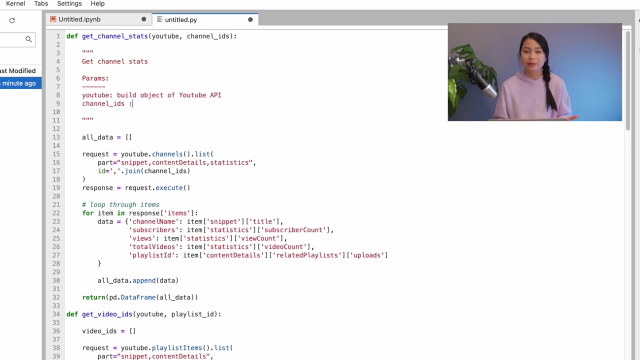 It's also a very good practice to move all the functions you made to a separate Python file and then later import this Python file to our notebook. This would make our notebook much cleaner and if you have time, you can also go into each function and write some documentation for it, just to help other people know what the function. 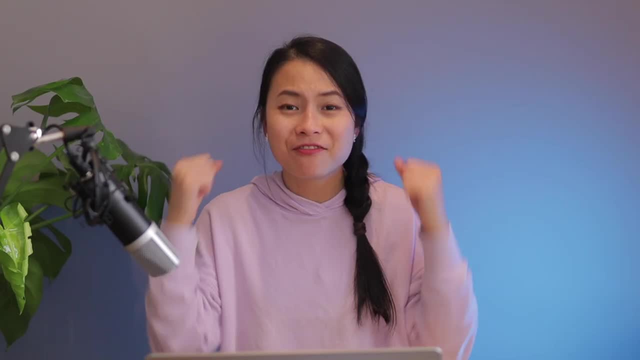 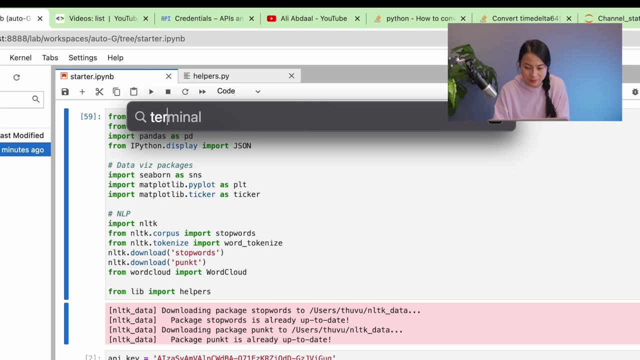 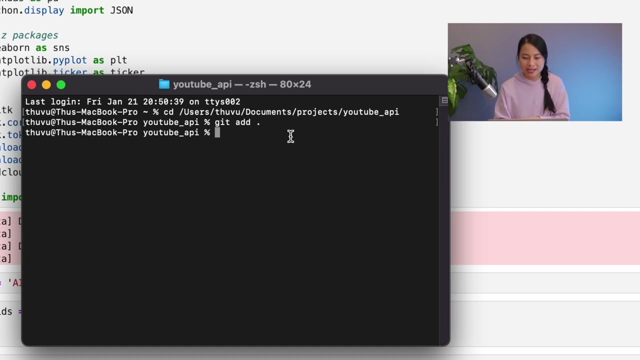 does and can easily reuse your code later on. finally, the last thing we want to do is to push this project to our current github portfolio. let's go to the terminal and run git add. this would add all the files in our folder to git, and then we can commit this change by typing git commit.